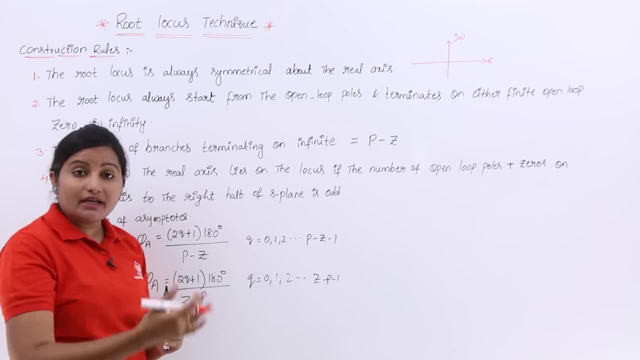 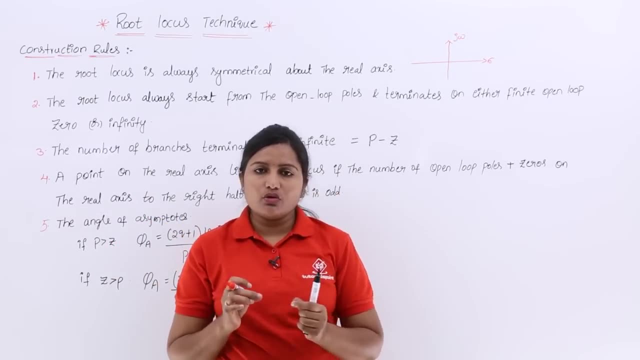 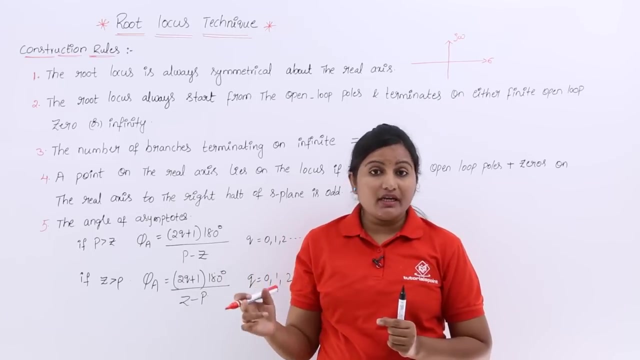 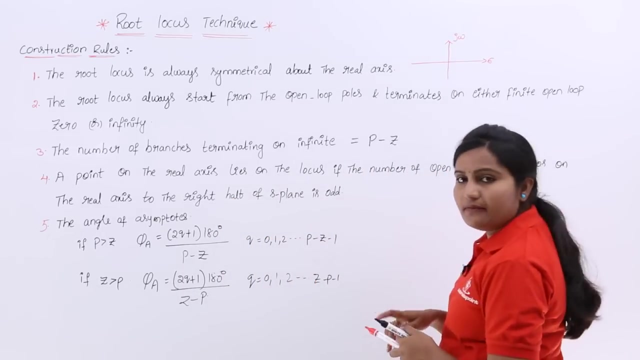 always starts from the open loop pole and terminates at finite open loop 0 or infinity. Generally, the root locus: the root locus always starts from open loop pole and terminates or ends at finite open loop 0 or infinity. That means here, for example, if you are having 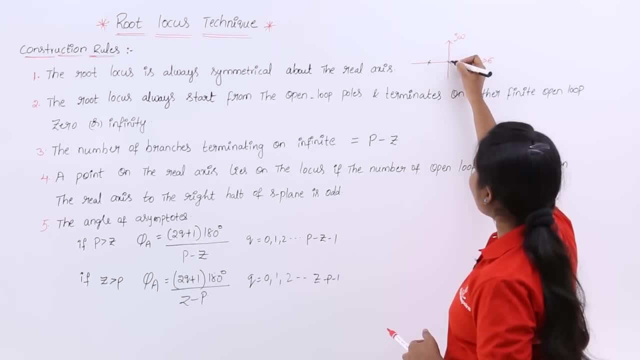 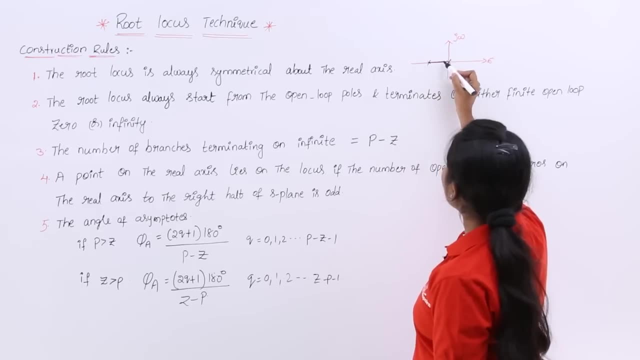 poles like this. if you are having poles like this, So here, for example, you are having root locus like this, symmetrical, about real axis, For example, if you are having any zero, here, your root locus, your root locus may start. 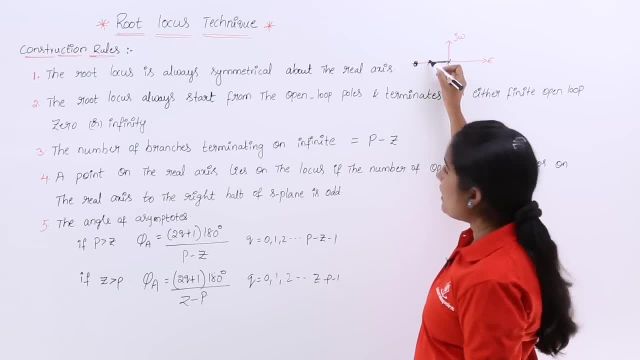 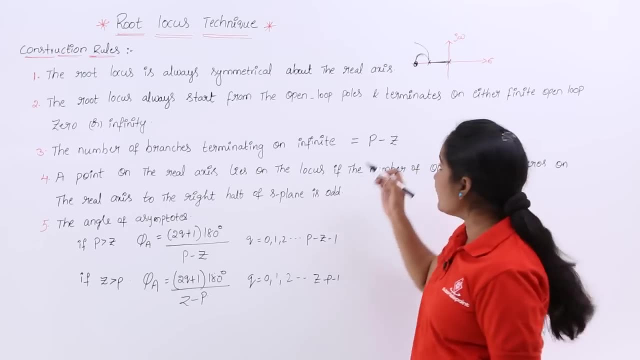 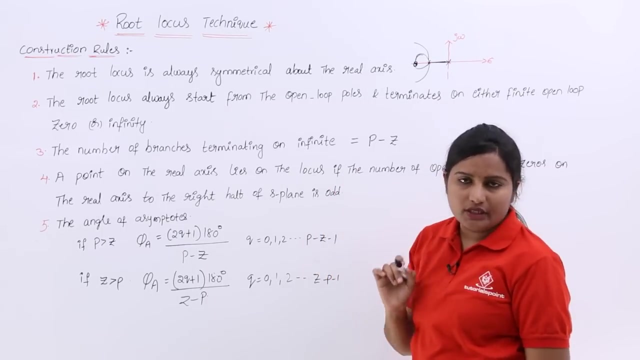 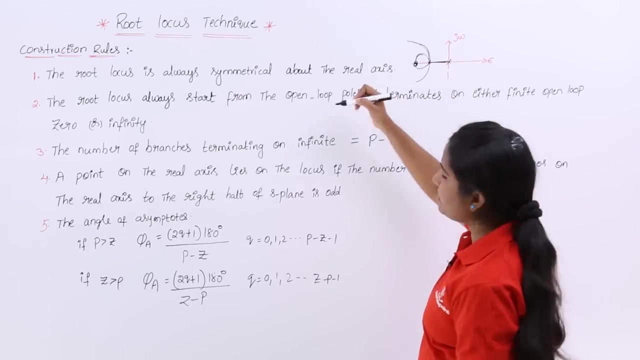 from here, any open loop pole, it may end at open loop 0, or it may terminate at infinity, like this or like this. It may terminate at open loop 0 or it may terminate at infinity. So here, if you see, so it is going to terminate at infinity. we do not know the end of that, whatever the root locus, we. 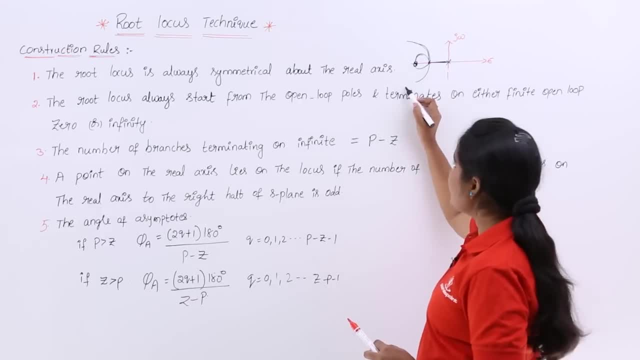 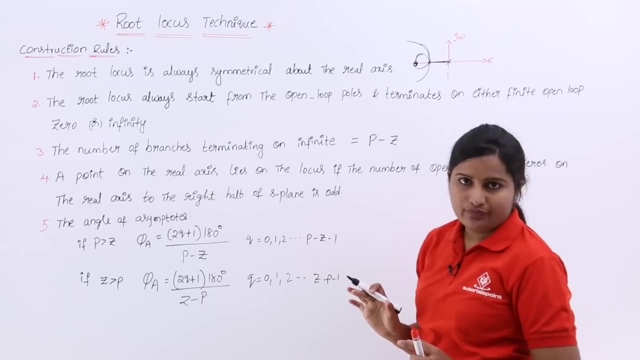 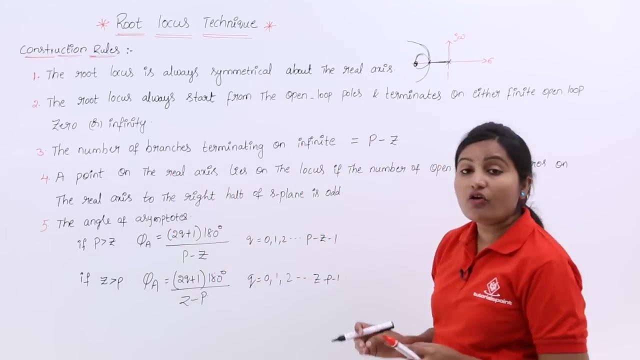 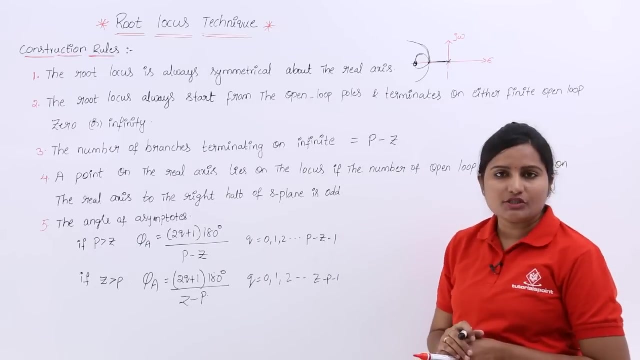 drawn. we do not know the end of that, so in this case, So this may terminate at infinity, or this may terminate at open loop 0. So here the number of branches terminating on infinity, the number of branches terminating at infinity is equivalent to p minus z, where p is the number of poles. 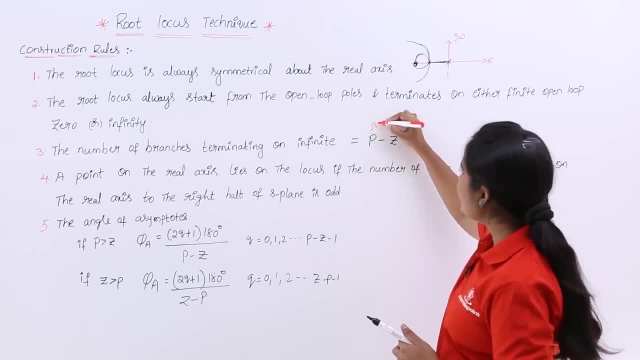 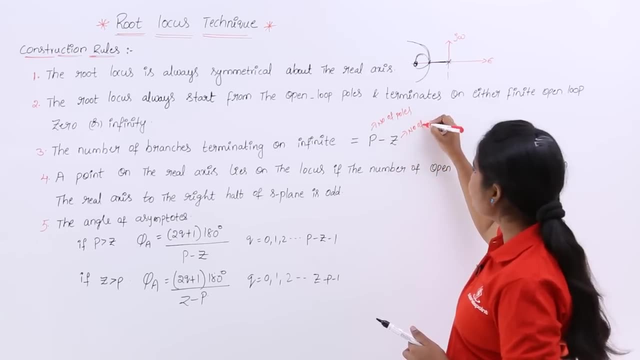 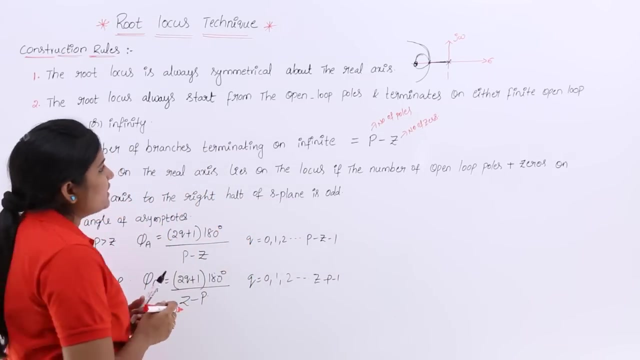 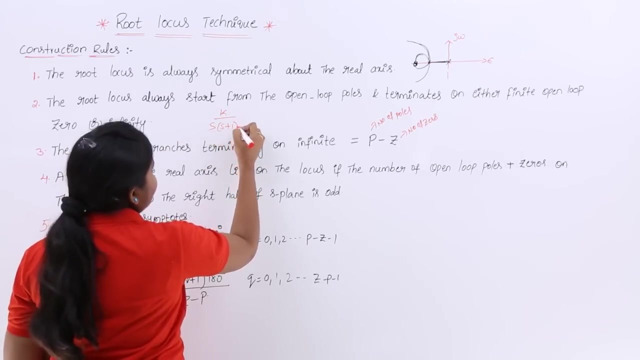 and z is the number of zeros. So this is number of poles and this is number of zeros. That means, for example, if you are given with any open loop transfer function like this, k by s into s plus 1. So here how we can determine. 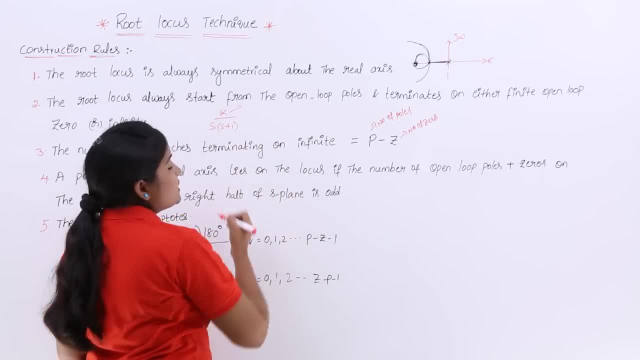 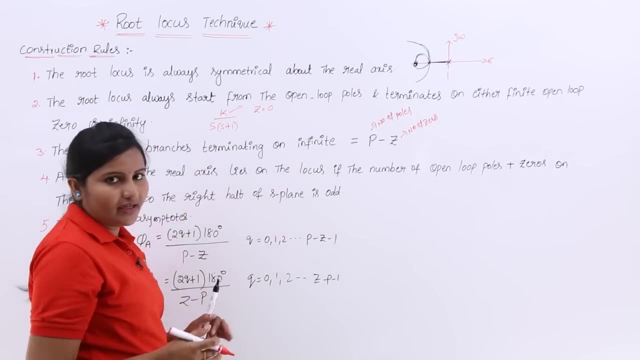 the number of zeros. So by observing the denominator we can determine the number of zeros. So by observing the denominator we can determine the number of zeros. So by observing number of zeros, here the number of zeros is equivalent to 0. why? because we are not having 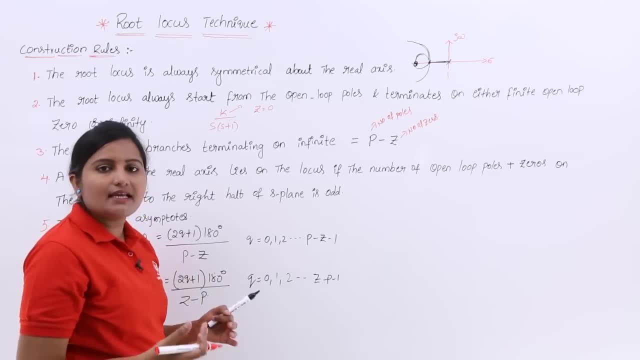 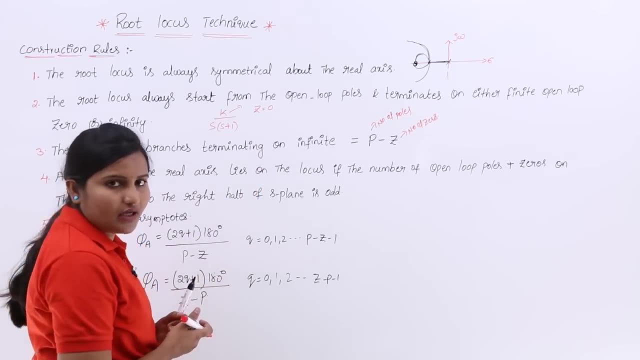 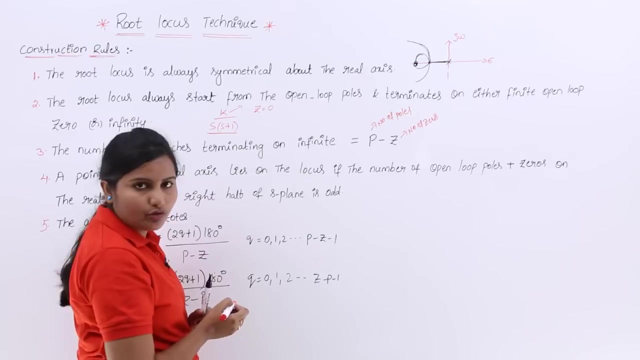 any s term. if you are having k into s plus 1, then s is equivalent to minus. 1 is the 0 in the numerator. so here we are not having anything. so number of zeros is equivalent to 0 and here the number of poles is equivalent to s equivalent to 0 pole, s equivalent to minus 1 pole. so totally. 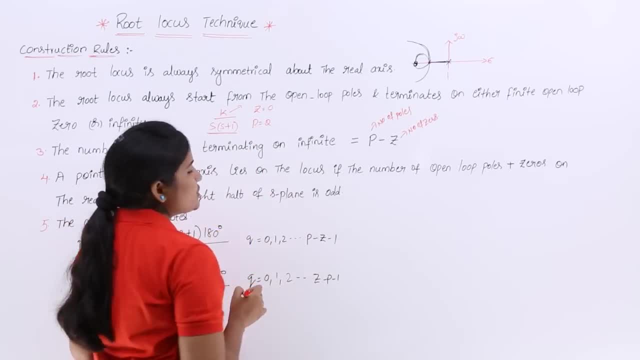 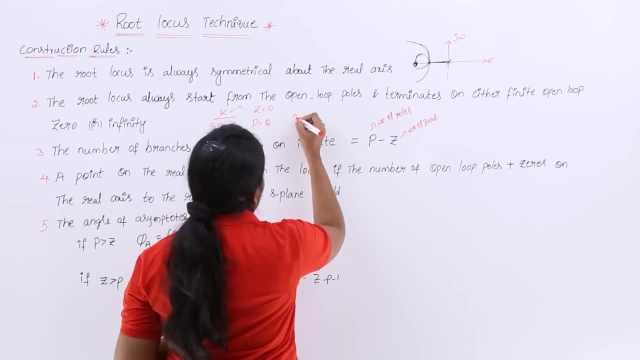 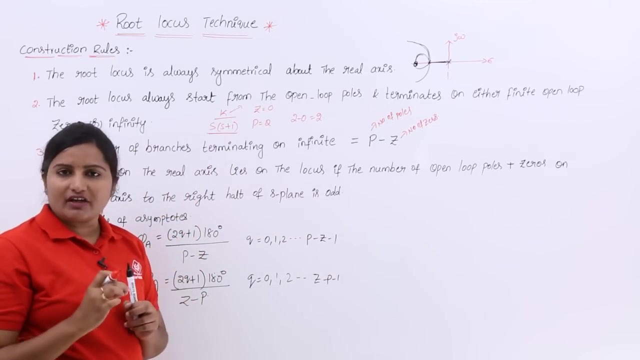 you are having, number of poles is equivalent to 2, so the number of branches. so here the number of branches is equivalent to 2 minus 0 is equivalent to 2. so here we are having one condition actually, whatever the branches that are going to terminate at open loop, 0 or 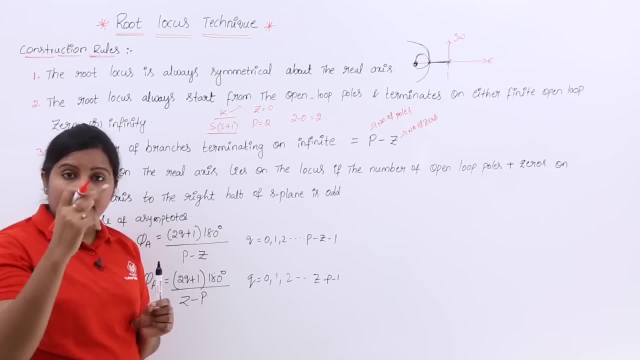 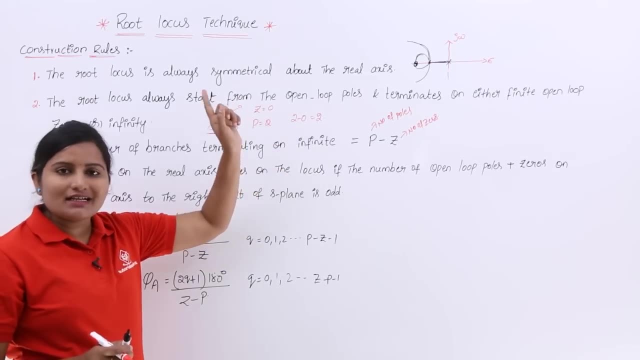 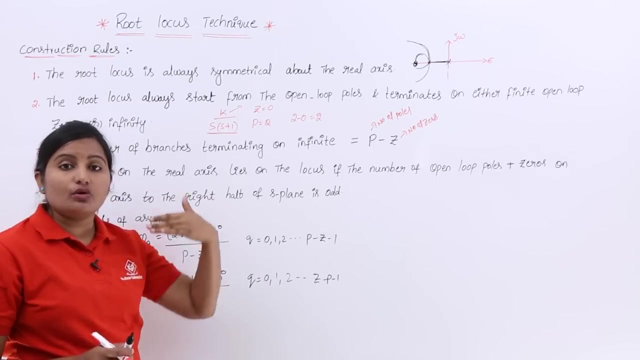 what are the branches terminating at infinity? 0. for that we are having condition, that is, if poles are greater than zeros. if poles are greater than zeros, then your branches are going to terminate at infinity. if zeros are greater than poles, then your branches are starting at infinity. 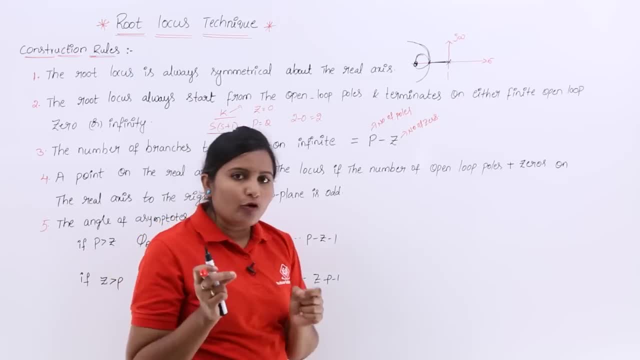 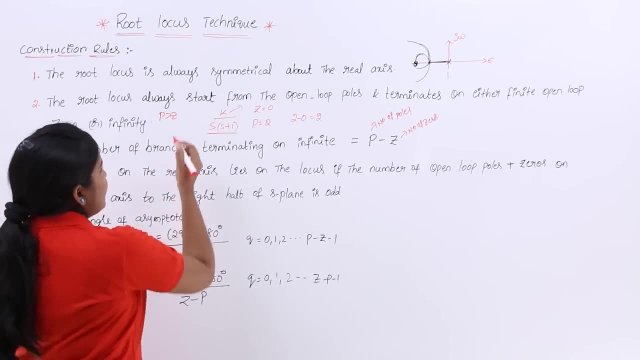 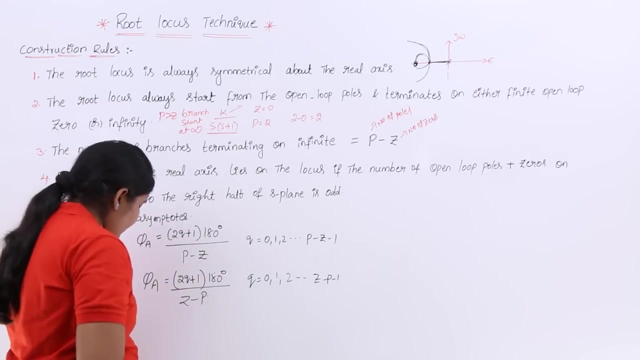 so you can observe the difference. if pole is greater than than 0, that means so if pole is greater than 0,, then branch start at branch start at infinity, not start branch terminates at infinity. So whenever poles are greater than 0's. 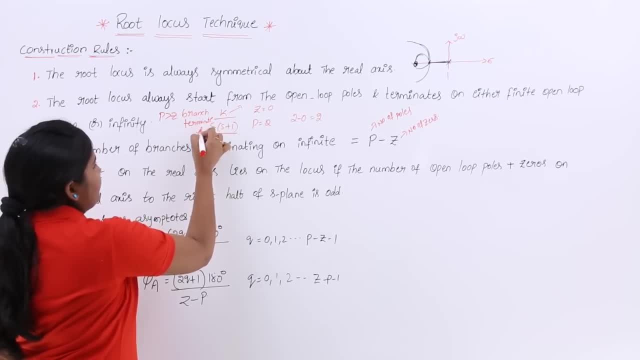 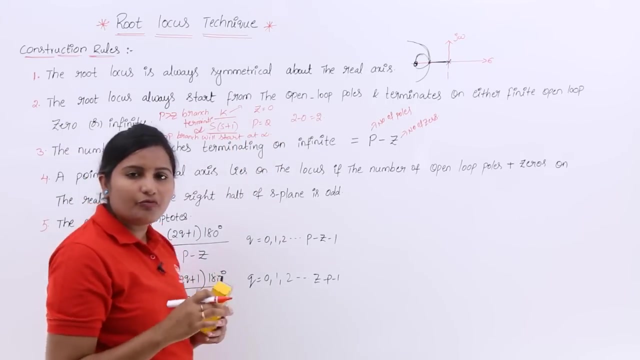 so branch will terminate at infinity. If 0's are greater than poles, then branch will start at infinity. branch will start at infinity. So this is the difference between the number of poles and 0's How the branch is going to vary. If poles are greater than 0's, then 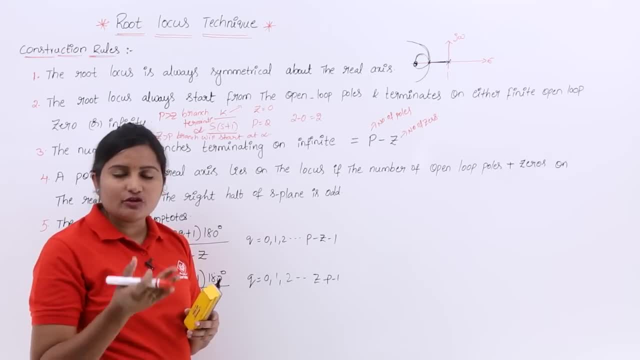 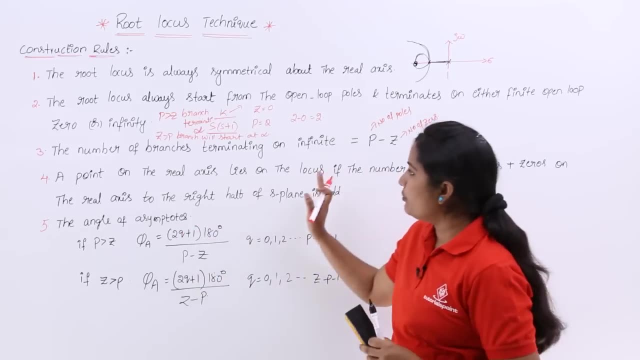 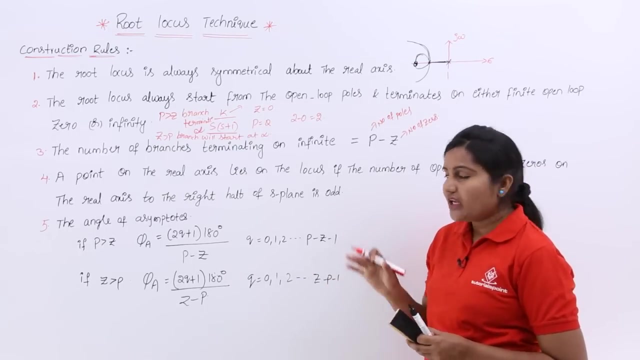 branch is going to terminate at infinity. If 0's are greater than poles, then branch is going to start at infinity. Now coming to very important fourth point, a point on the real axis lies on the root locus. if the number of open loop poles plus number of open 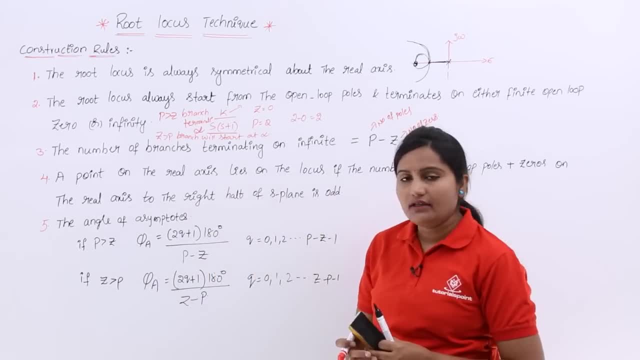 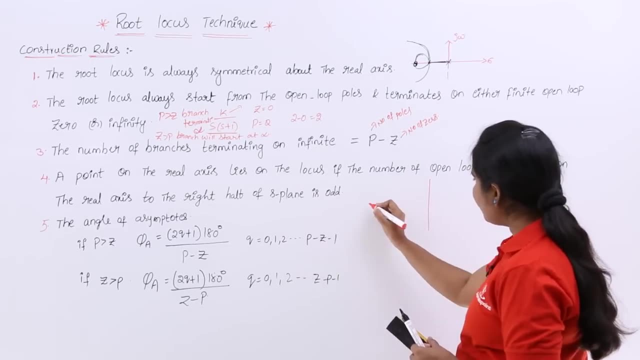 loop 0's on the left half of S plane must be odd. So that means, for example, you are having, you are having a point on the left half of S plane. so that means, for example, you are having a point on the left half of S plane. so that means, for example, you: 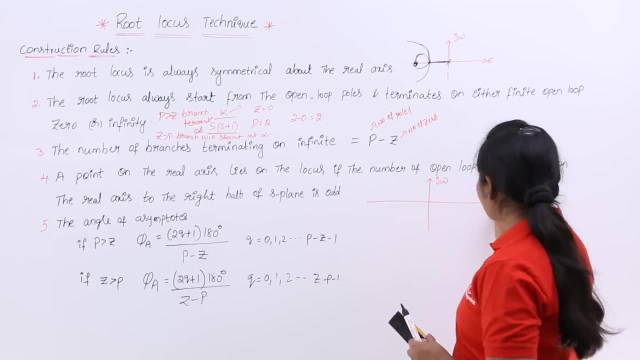 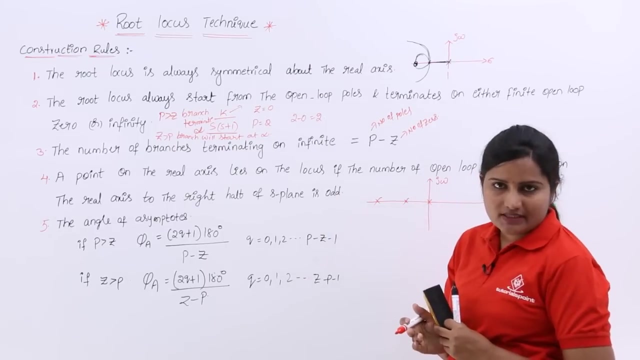 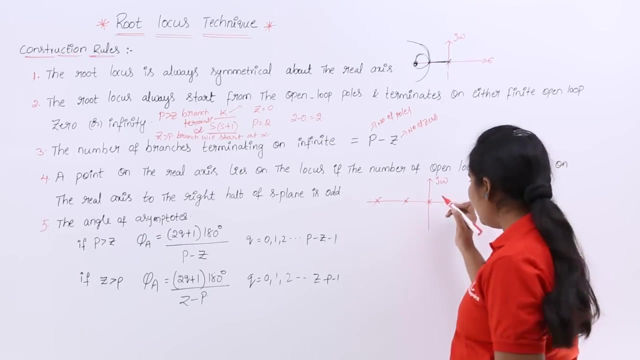 are S plane like this j omega axis, and this is real axis, You are having 3 poles at origin one pole and here is one pole and here is one pole. So here to the left half of S plane, your number of poles plus 0's must be odd. For example, here, from here to here you can. 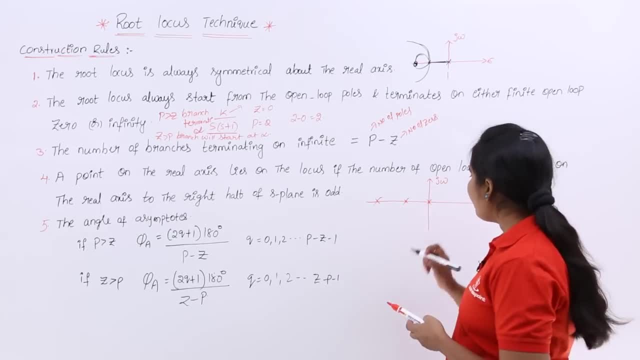 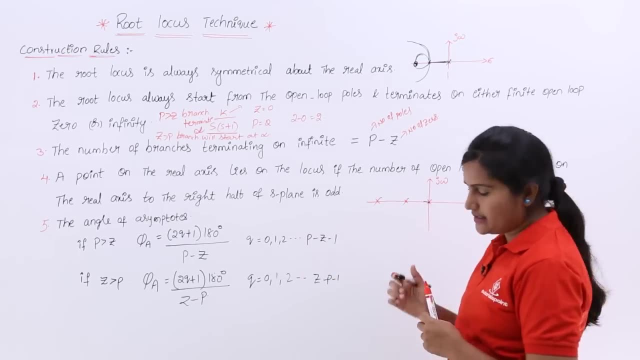 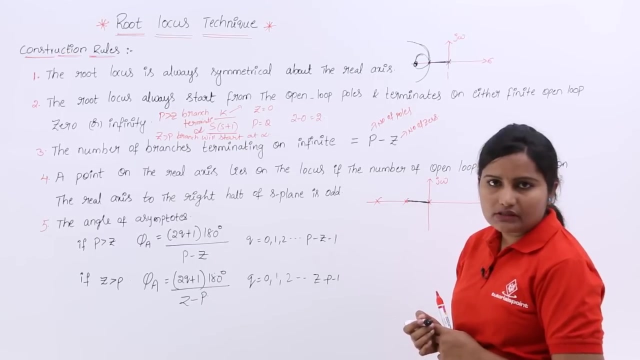 observe only one pole. Observing only one pole is nothing but odd. From here to here, my root locus is symmetrical about real axis, So here I am having root locus Whenever this pole started, then my poles count is total. number of poles are 0's count is increased to 2.. When you are hearing, 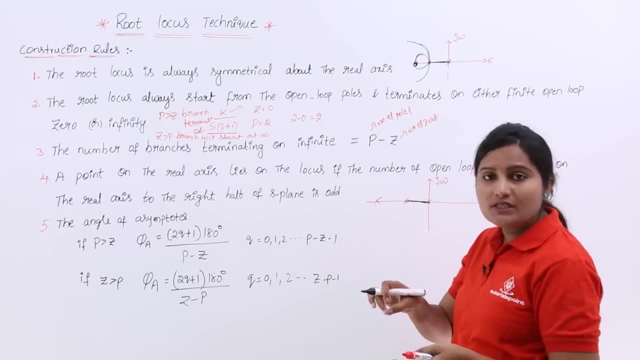 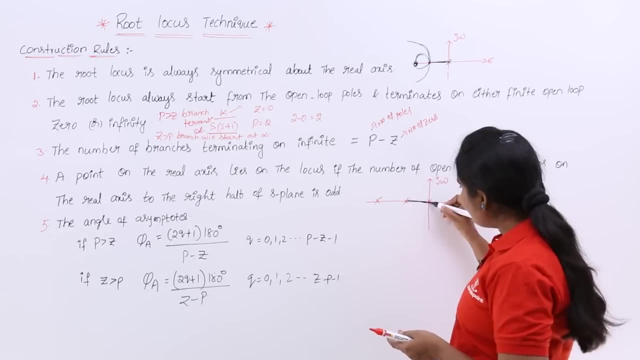 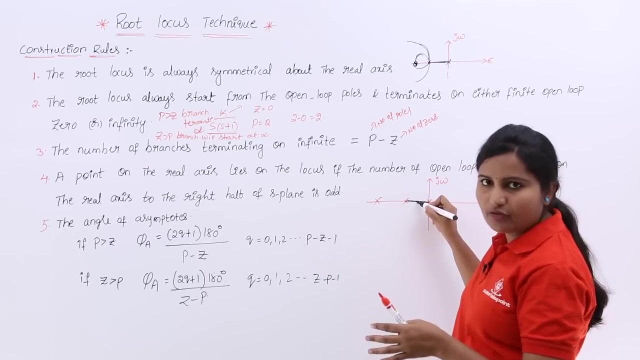 0's count is the even number, Always the open loop poles plus 0's must be odd. to write the, to draw the root locus. So I am just moving in this way. So in this point, if anyone asked you how many poles are there in your path, So only one pole. So after crossing, 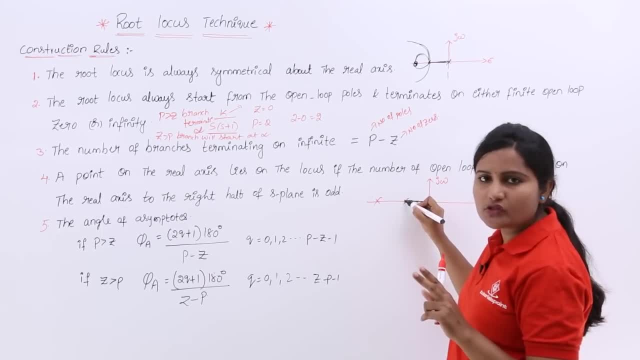 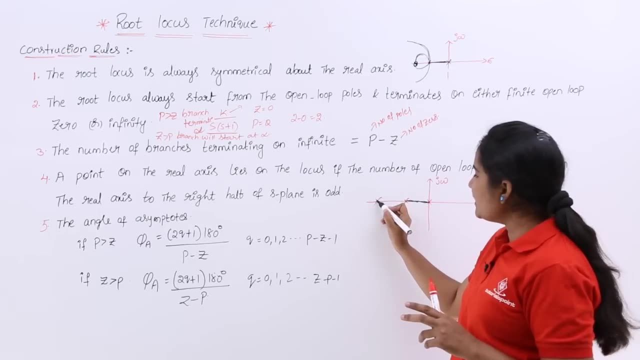 this pole. how many poles are there? means we are having 2 poles. So here you are not going to consider the root locus in this position After crossing this pole. so again you will get root locus. Why? Because the number of 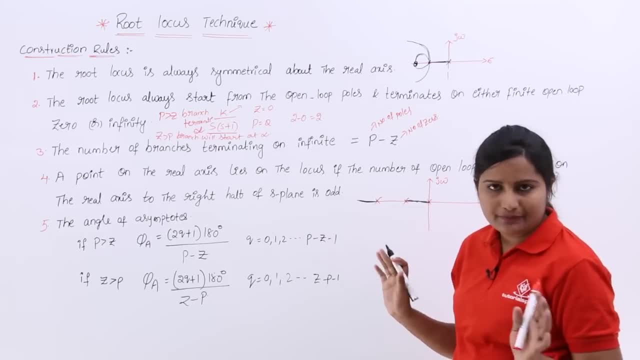 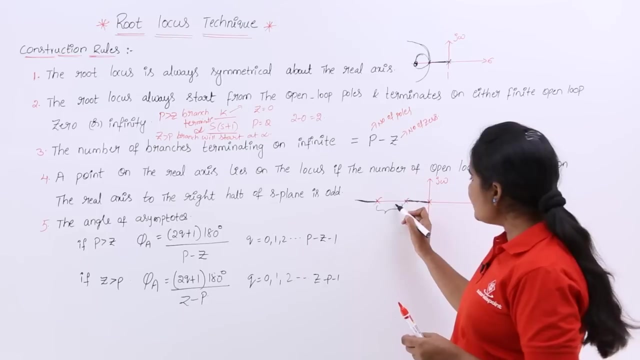 poles from here is 1 plus 1 plus 1, 3.. So totally 3 poles will be there. So here this part would not come because the addition of open loop poles and 0's, So in this position 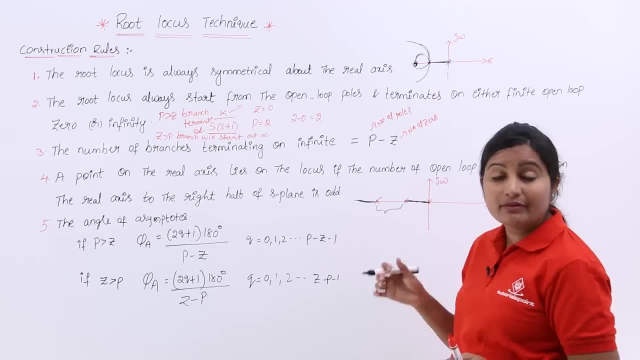 from origin is equivalent to 2.. So here you are having root locus. So here you are having root locus. So here you are having root locus. So in this position, from origin is equivalent to 2.. So it must be odd, not an even value. but here, in this position, the number of poles. 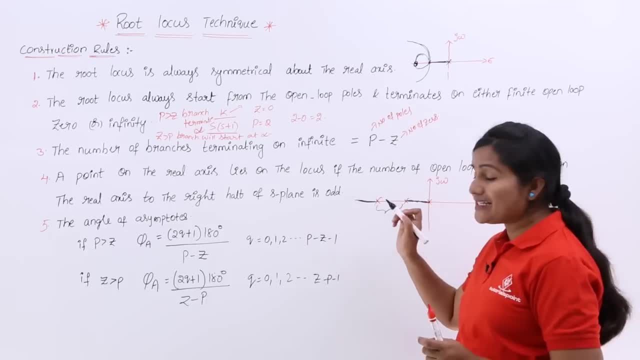 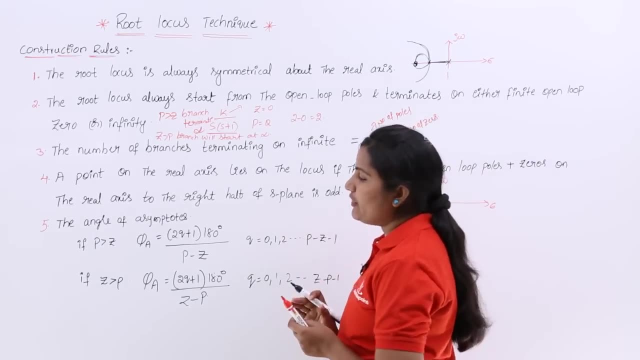 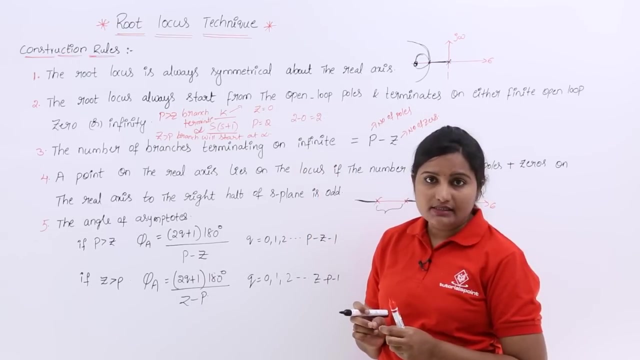 plus 0's is equivalent to 2.. That is why we are not considering that position. So that is the meaning of this point. After that, the angle of asymptotes. So whatever the branches we are taking, that branches, angles are nothing but asymptote angles. So here, if p greater, 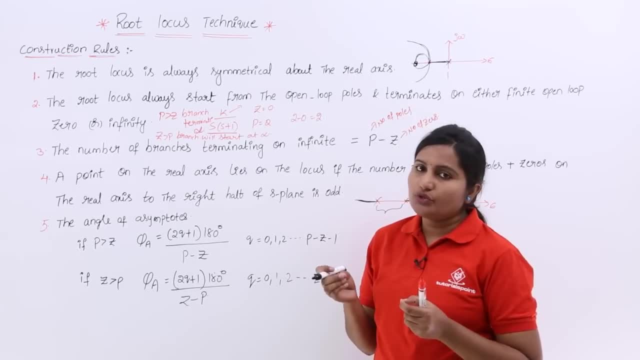 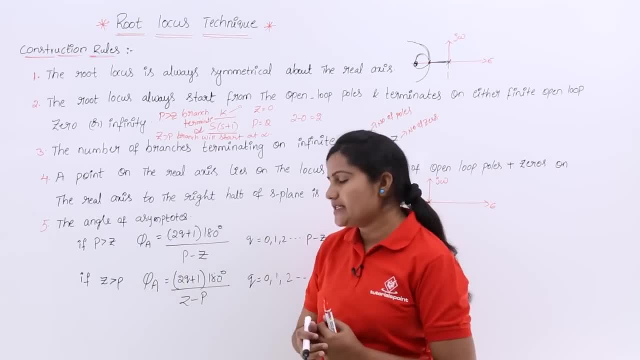 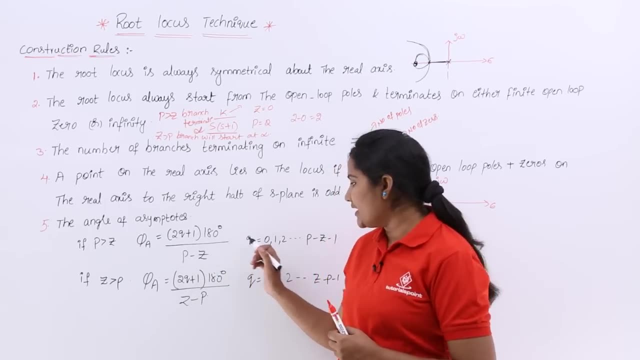 So the asymptotes angles are: phi: a is equivalent to 2, q plus 1 into 1, 80 divided by p minus z, where q is equivalent to 0,, 1, 2, so on p minus z minus 1.. And if z greater than p, 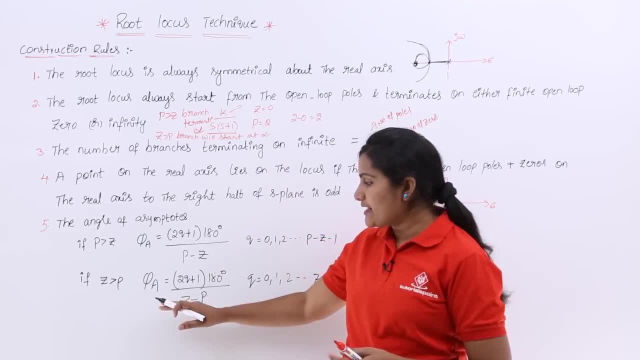 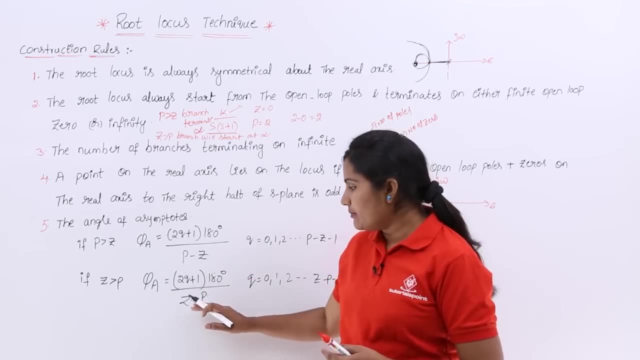 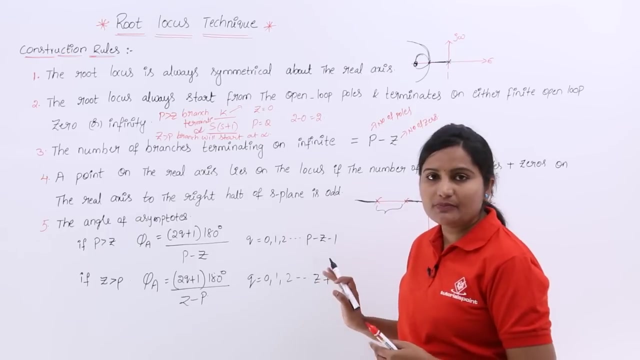 the branches. their given term is going to be the opposite. therefore, p is going to be is. we will start at infinity. and the asymptote angles are: phi: a is equivalent to 2, q plus 1 into 180, divided by z minus p, So where q is equivalent to 0, 1, 2, so on z minus p. 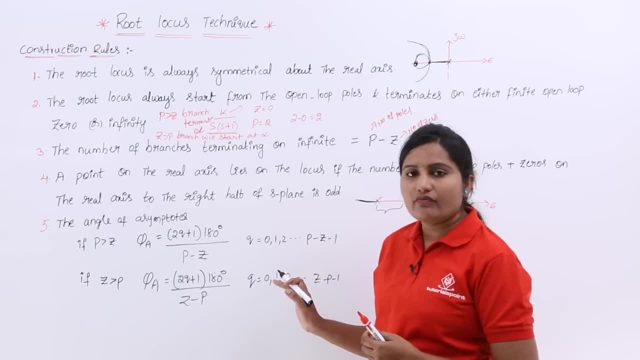 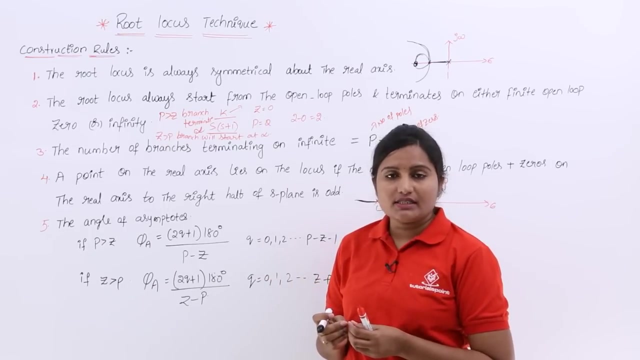 minus 1.. So this is very, very important conditions we need to follow when you are writing root locus. Some more conditions are there that we will discuss in the next slide. that means so what is the centroid we need to consider and what is the angle of departure and angle? 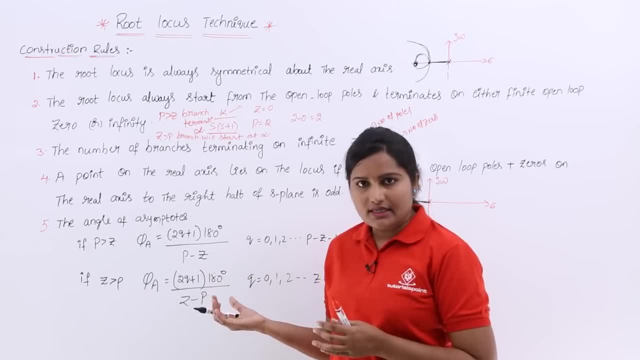 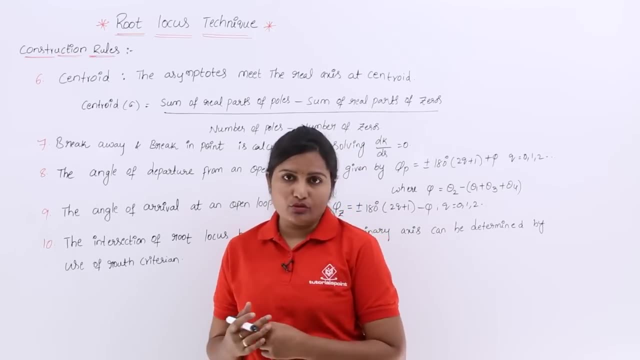 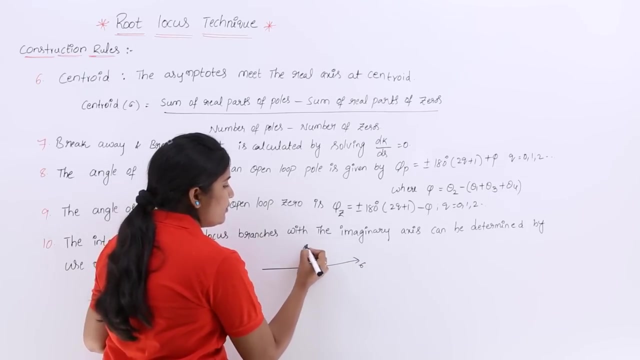 of arrival that we will see in the next slide in the same video. In previous 5 points we discussed points about root locus. that means construction rules for root locus, as So root locus is symmetrical about real axis. that means the first 5 points. in the first 5 points we discussed the root locus is symmetrical about. 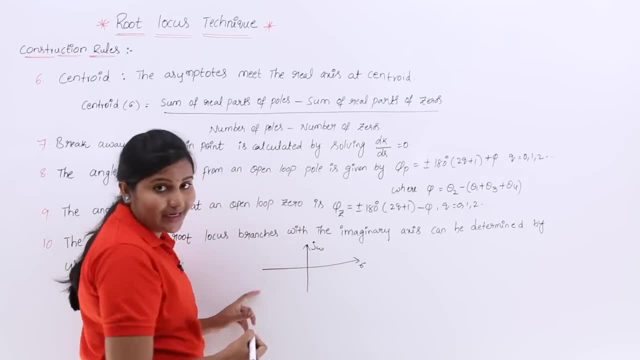 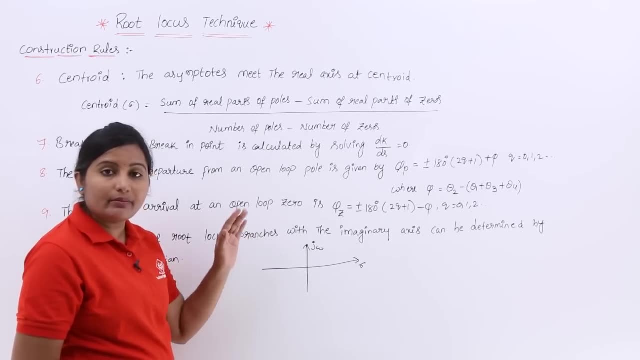 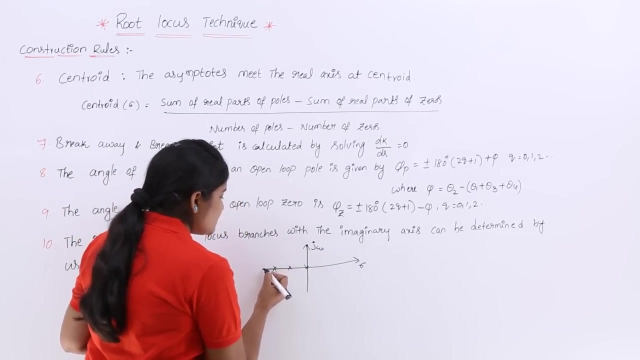 real axis, that means so it is symmetrical to real axis and after that. So always root locus starts at open loop poles and terminates at open loop 0 or infinity, For example. if you are having poles like this, it may starts at open loop pole, any open loop pole, it may. 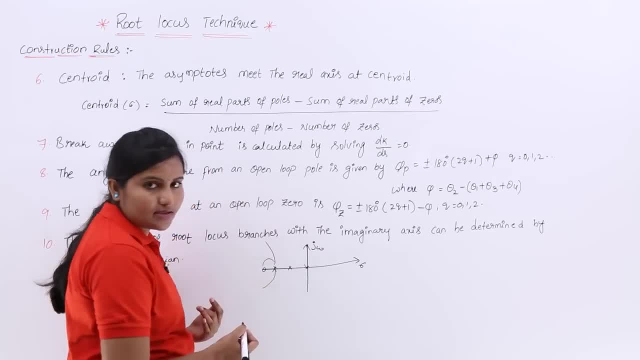 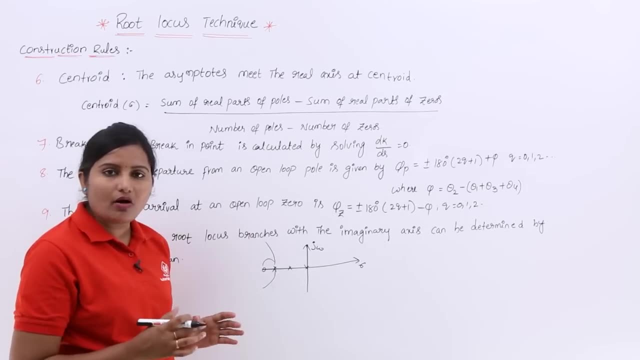 terminate at 0 or it may terminate at infinity. So if you have poles like this- and another point, we discussed that a point is said to be on root locus whenever this sum of open loop poles plus 0's must be odd, that means 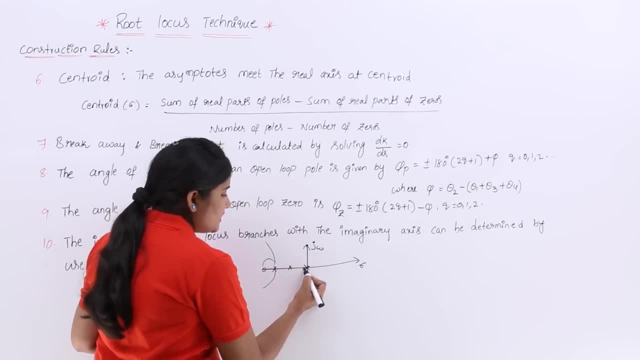 so here, if you are having 3 poles like this, So in this root locus path so up to here, there is only one pole from origin. from here onwards we can say we are having 2 poles. So that means when you are moving to this side in the back section how many poles are? 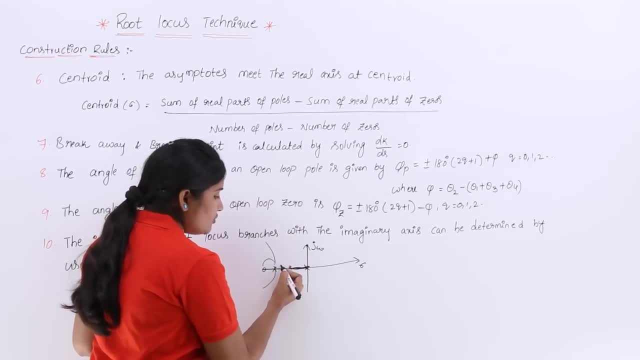 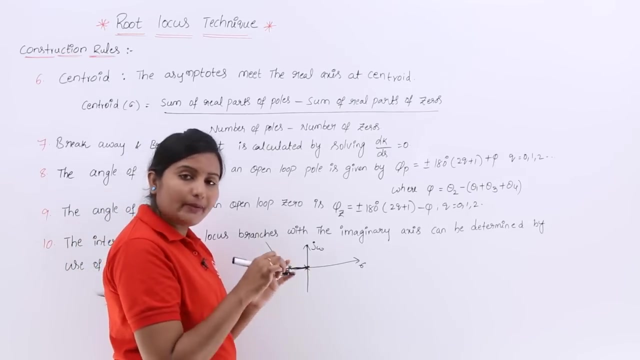 there means we are having 2 poles. that is why we are not going to consider this section and the coming to here. from this pole onwards, the number of poles will be 3 again. that means from the origin moving towards minus infinity region. the number of poles plus 0's must be: 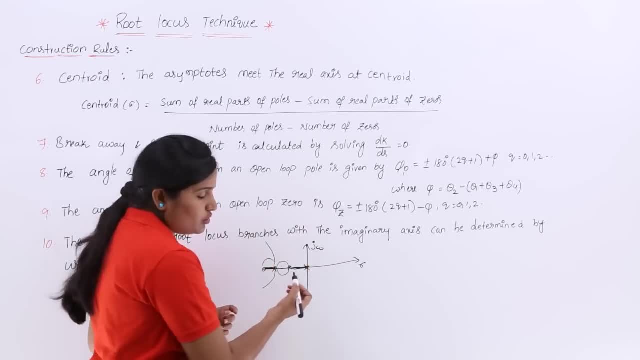 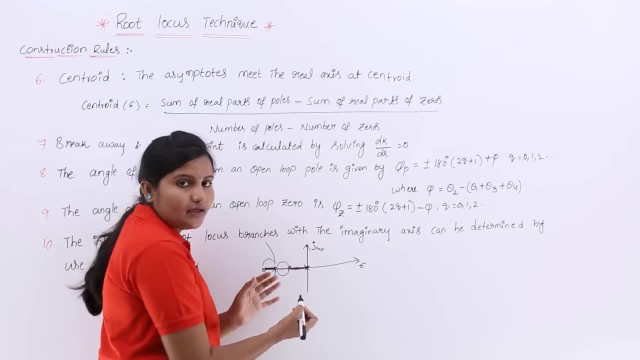 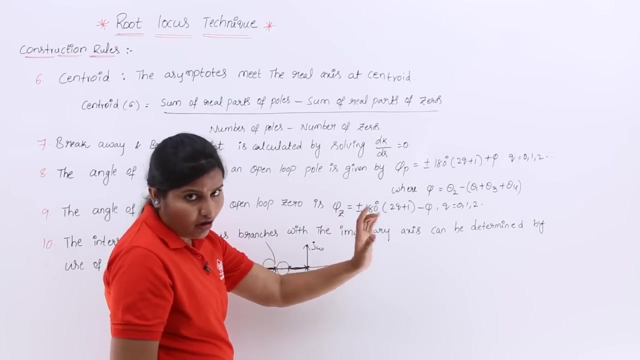 odd to write the root locus or to draw the root locus here. I am having root locus here, but I am not having here that why? because how many number of poles plus zeros are there in the? in the way of that origin means we are having. 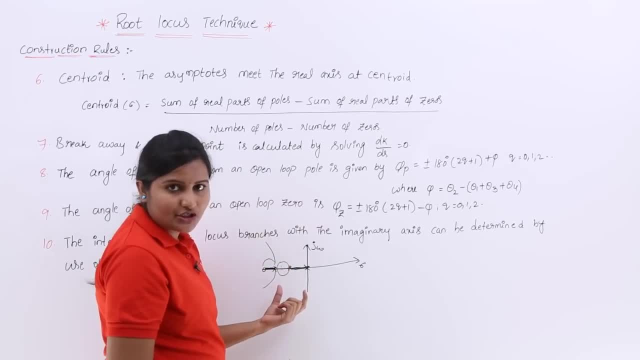 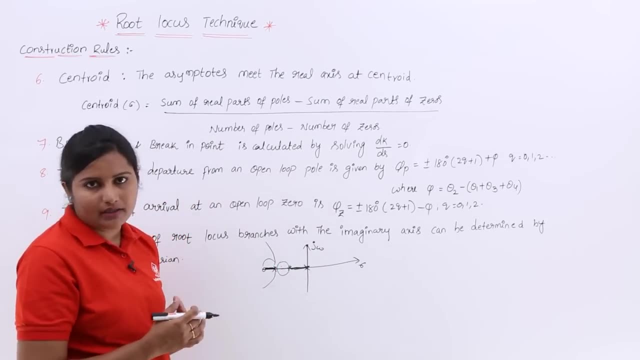 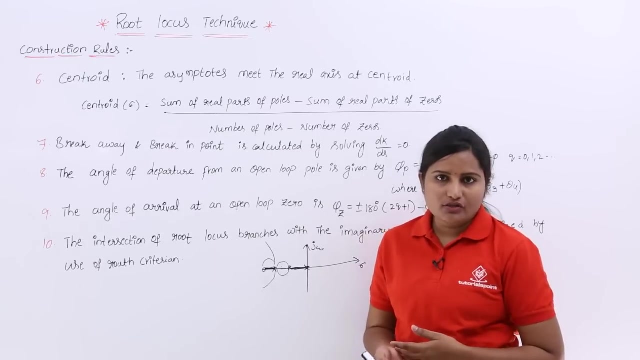 two poles. that is why I am not taking that condition, I am not taking that region. why? because my number of poles plus zeros must be in odd number and coming to poles and zeros. so if poles are greater than zeros then the branches will terminate at infinity. zeros are greater than. 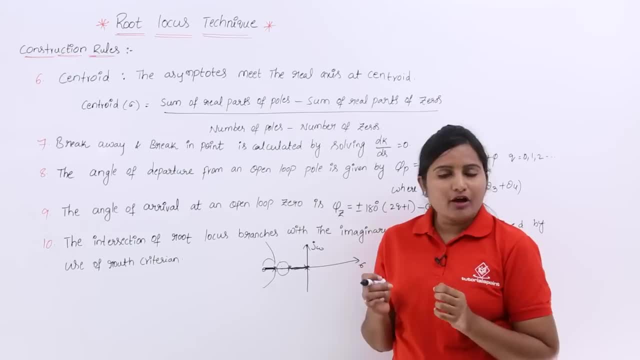 poles, branches will start at infinity. and one more important point is: for example, if branch is terminating at infinity, then we can say: a zero is there at infinity. if a branch is starting at infinity, that is the meaning: a pole is there at infinity. so that is very, very important points. 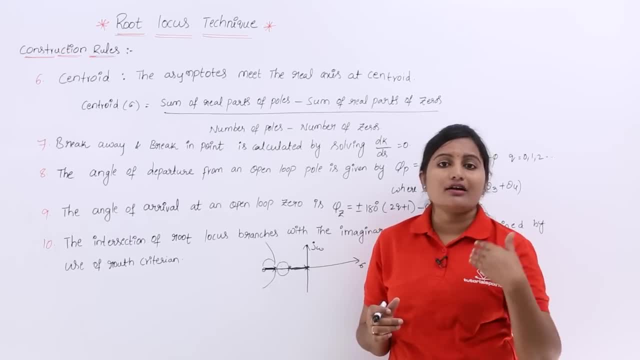 if your saying your branches are terminating at infinity. terminating at infinity means so that implies a zero is there at infinity. if your branches starting at infinity, that means if zeros are greater than poles, then you are said to be your branches are starting from infinity. so we can say: 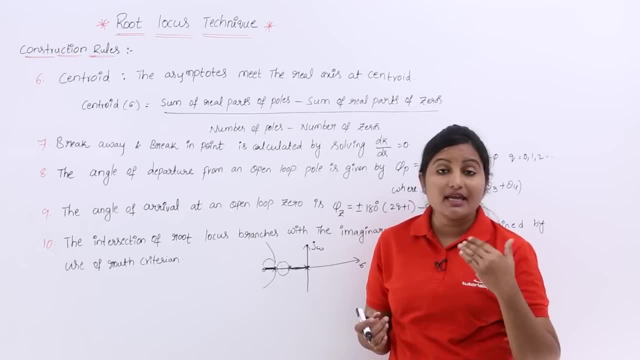 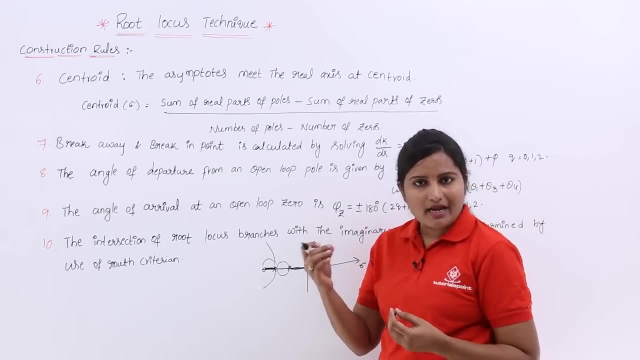 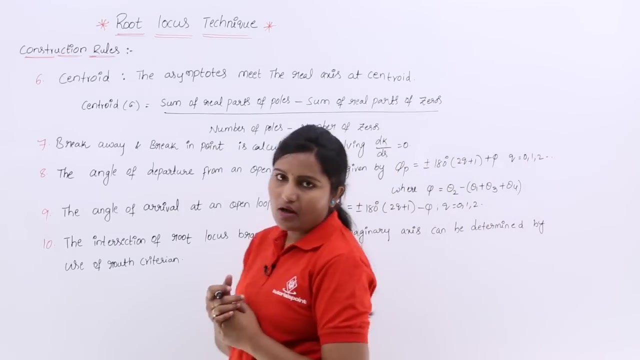 if, the if branches are starting at infinity, we can say: a pole is there at infinity, why course So? always your root locus branches starts from poles and terminates at zeros. So that is why we given that clarification and now here coming to this centroid. Centroid is: 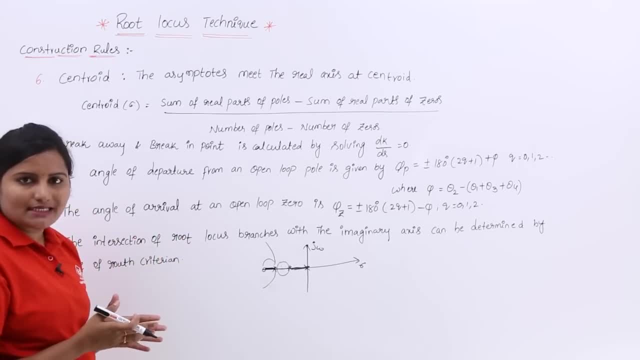 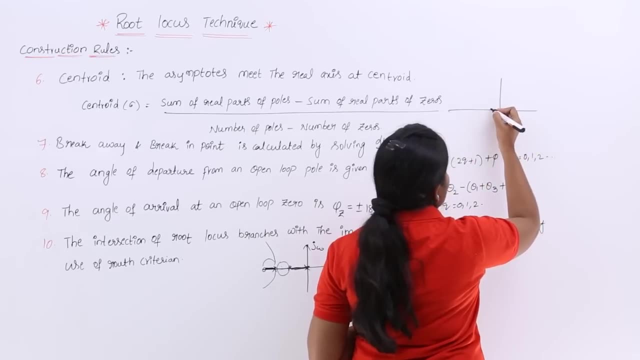 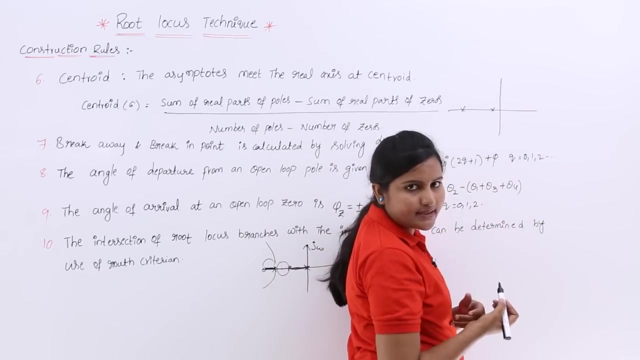 nothing but meeting point of your branches or asymptotes in the real axis. So here, for example, if you are having root locus like this, if you are having so poles like this, So you are having asymptotes 4, asymptote, 3, asymptotes, So that asymptotes will meet at centroid in the real 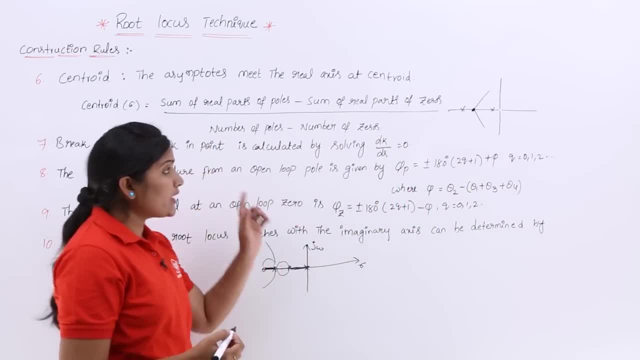 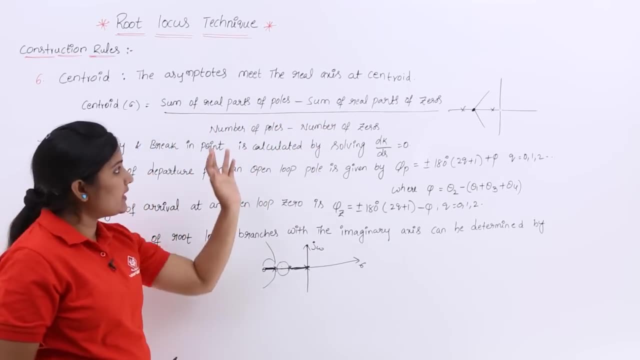 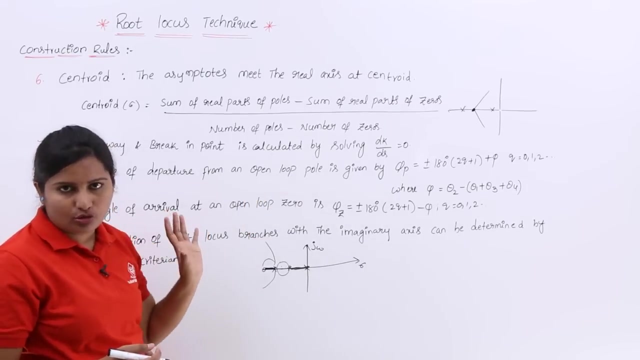 axis. So this is the centroid. So the to calculate that centroid, the formula is sum of real parts of poles minus sum of real parts of zeros, divided by number of poles minus number of zeros. This is the formula to calculate the centroid for the root locus and coming to break away. 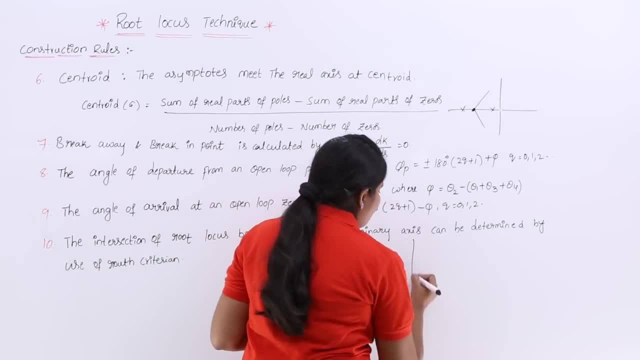 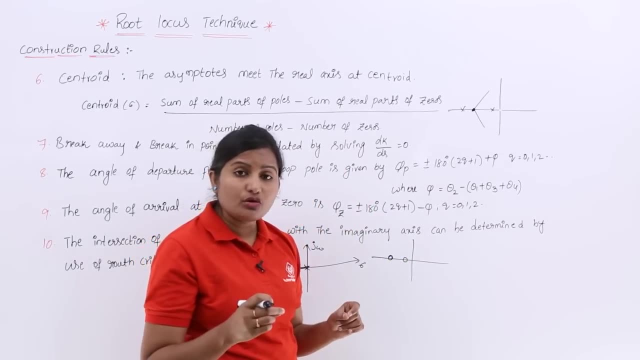 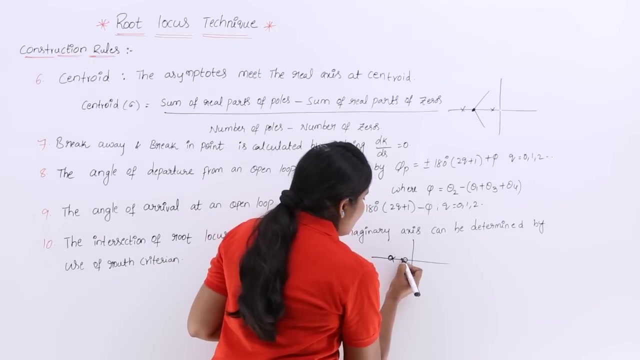 and break in points. So here I need to discuss one more point. So whenever you are having zeros, as I told you, always root locus starts from poles and ends it or terminates at zeros. So here this is going to terminate at zero. When zero is there an. 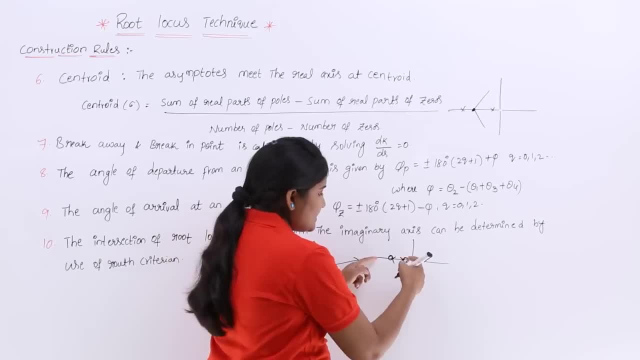 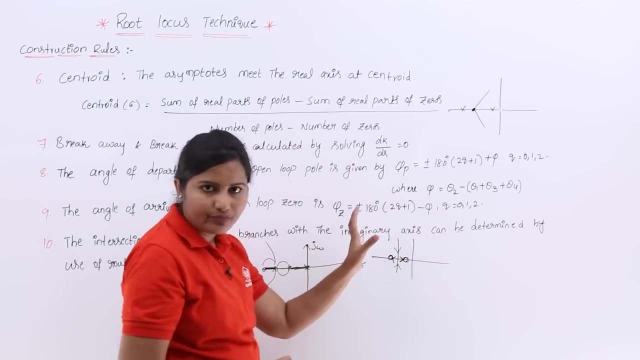 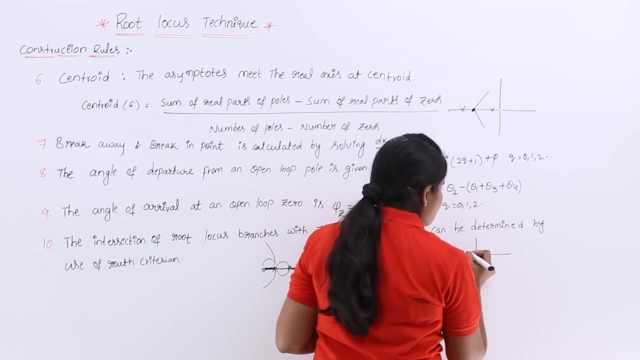 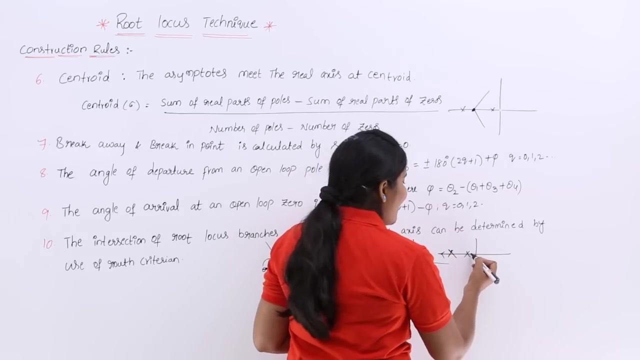 incompatibility Incoming arrow will be there. To get this incoming arrow, we need to have any break in point. So that means: like this or like this, we need to have that break in point. or in case of poles, For example, if you are having poles like this, from this poles we are. we need to draw away from poles. 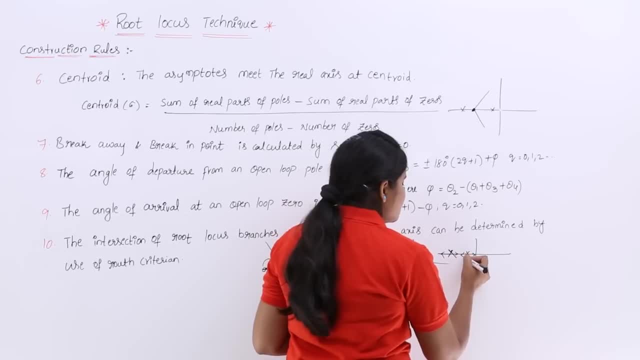 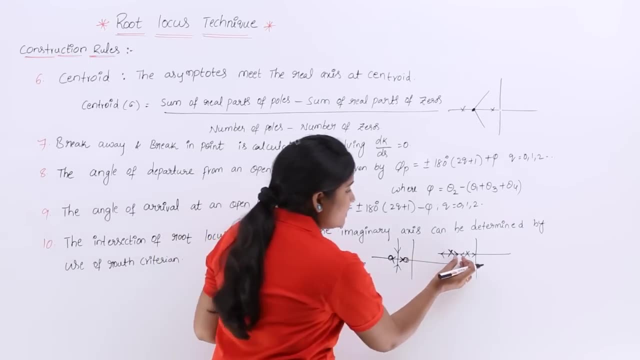 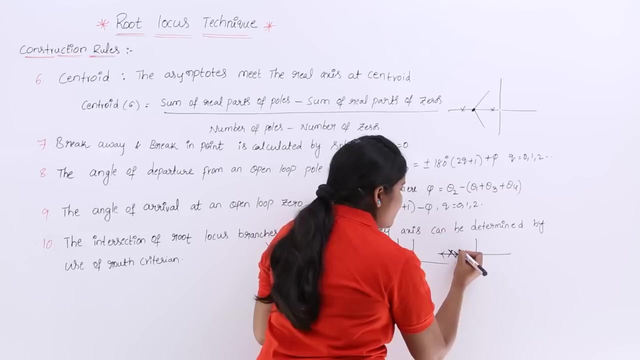 that means like this or like this, So we need to draw the arrow marks away from that poles. So here, when you are writing that arrow marks away from that poles, So this line may go like this or like this. so that means so by entering, like this, the direction. 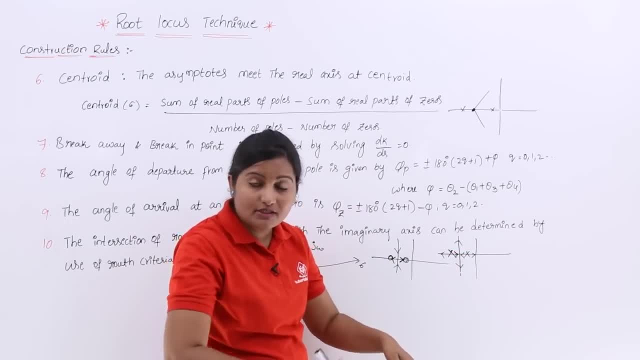 may be like this or like this. that means break away points. It is going away from poles here coming to here. this is going to the zeros. that means the arrow marks going to the poles. So this is like this: there you have drawn arrows going to the zeroes At the 0s. this is Ad how they. are the points between legislator also minus to 0, that they will be deducted right in this parallel lines. that means they are getting dealt with. that arrow marks. The arrows are able to be obtained in points getting томoetat primary or mini bind shown immediately. So theально. 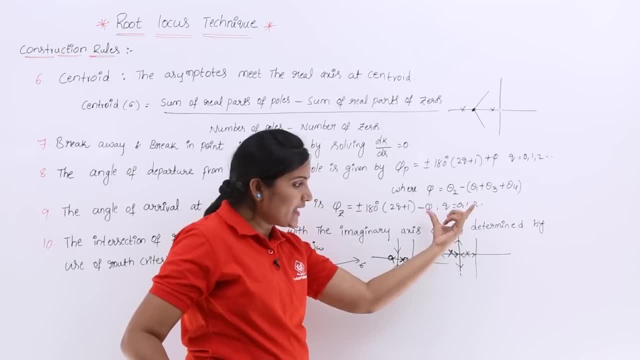 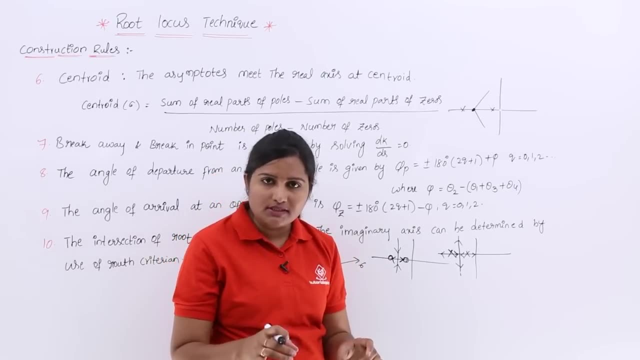 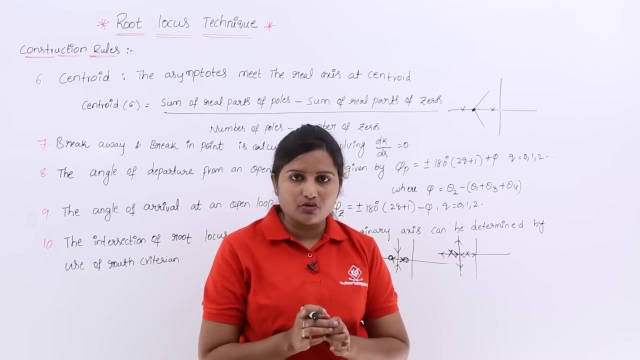 marks going into the 0s. here the arrow mark is going away from the poles. That is why, whenever you are having 2 poles, definitely we are having breakaway points. Whenever you are having 2 0s in between 2 0s, we may have break in points To calculate break in points. 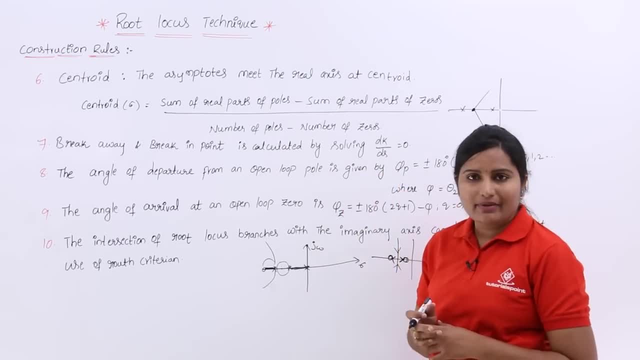 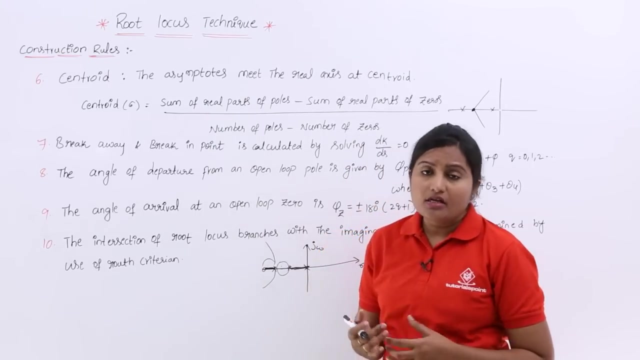 or break away points. so we need to have: dk by ds is equivalent to 0 condition. By solving dk by ds is equivalent to 0 condition. so we are going to get breakaway or a break in point. So now the angle of departure and angle of arrival. So when we will get this? 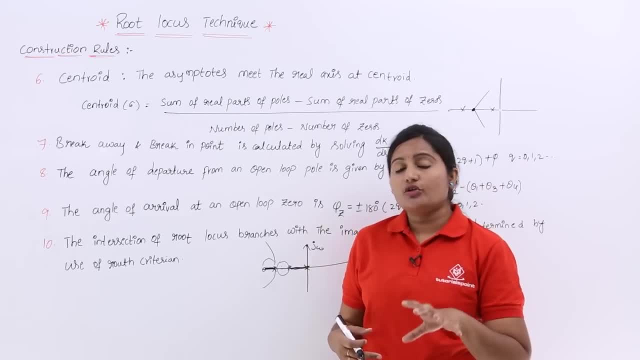 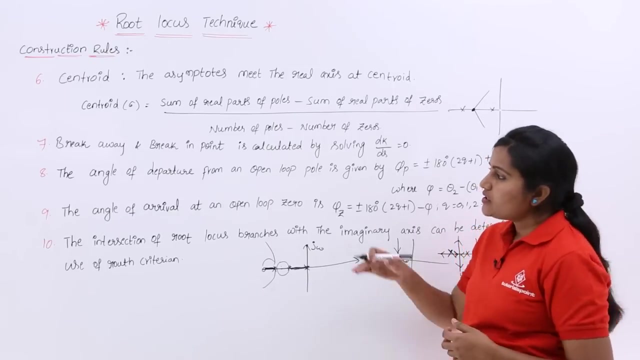 angle of departure and angle of arrival means whenever you are having imaginary roots, whenever you are having imaginary poles or 0s, then you are going to get the angle of departure and angle of arrival when you are having imaginary 0. So here the angle of departure from open loop pole is given by phi. p is equivalent. 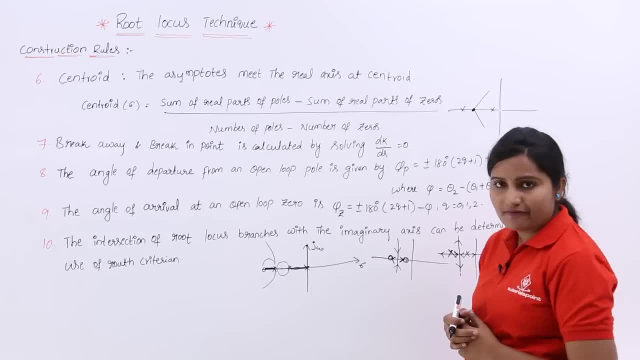 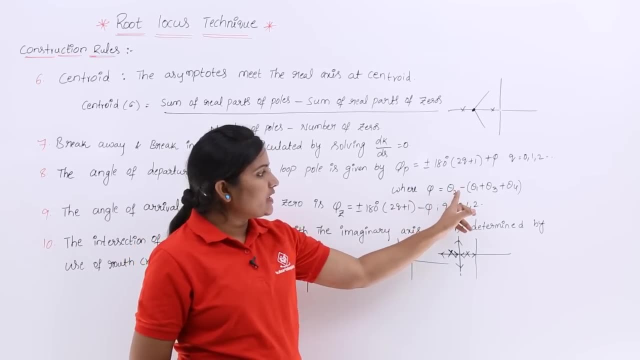 to plus or minus 180 degrees into 2 q plus 1 plus phi, where q is equivalent to 0,, 1,, 2,, 3 and so on. And here, where phi is equivalent to theta 2 minus theta 1 plus theta 3 plus, 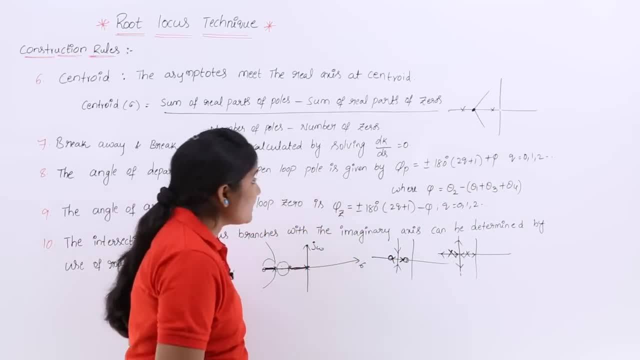 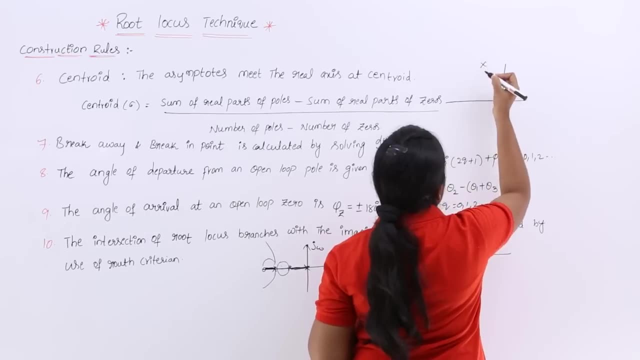 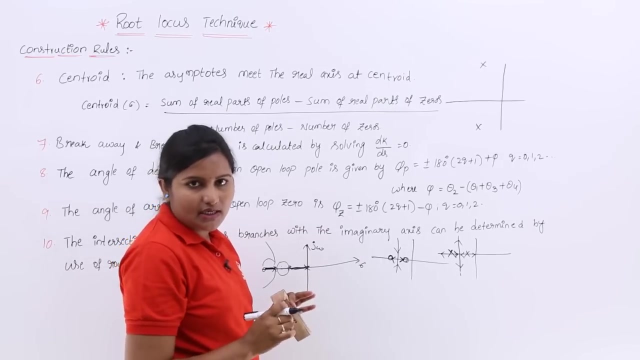 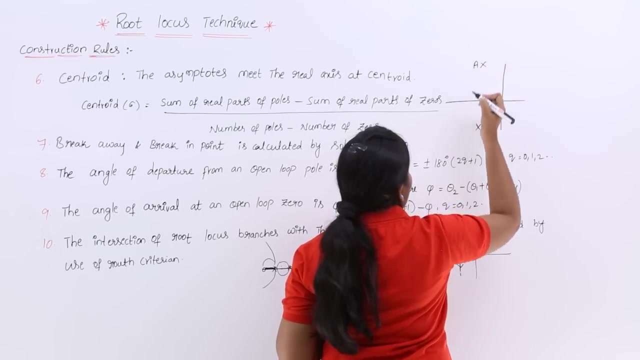 theta 4.. Why I given this equation means for this diagram I given this equation. please observe clearly: If, for example, you have imaginary pole like this, So if you are having imaginary pole like this, a plus j, for example, if you are having like this: So here this is a and this 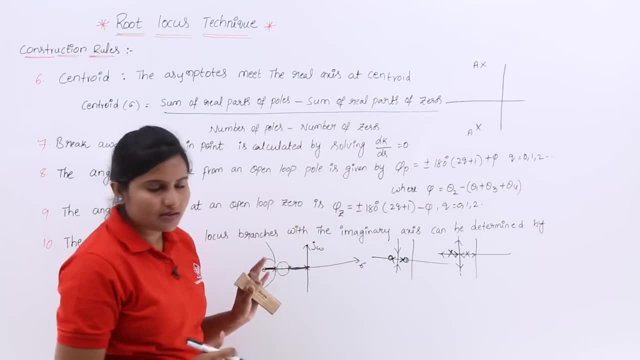 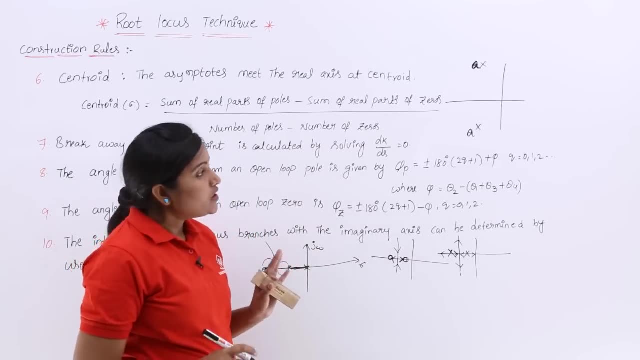 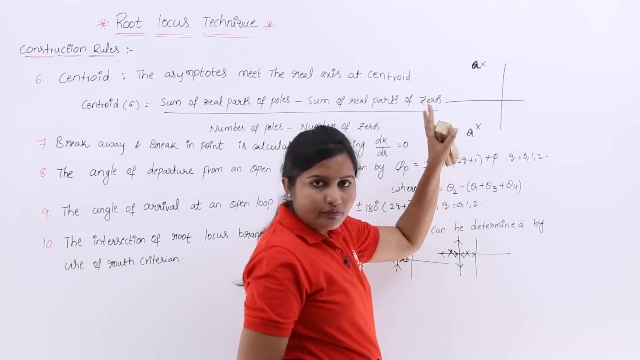 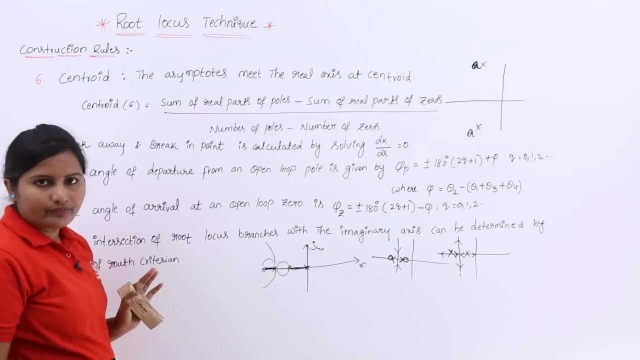 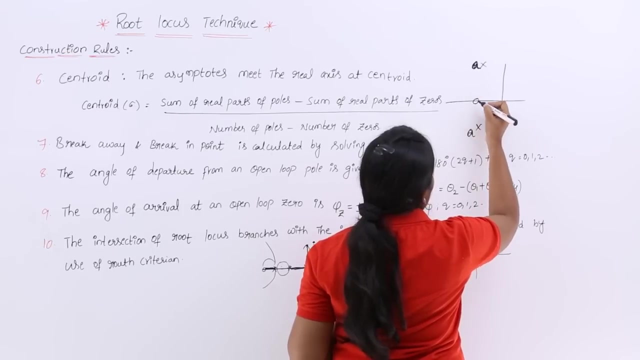 is a. So you, if you are having like this, this is your imaginary root, a. So now here, this imaginary root, a root, we need to calculate the angle of departure. Why? Because that is a pole. So angle of departure can be calculated like this: For example, if you are having a 0, like this and 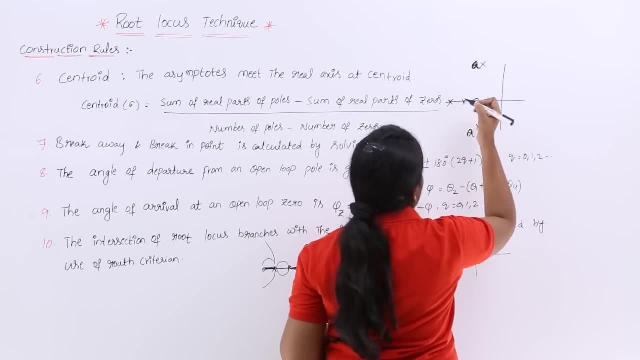 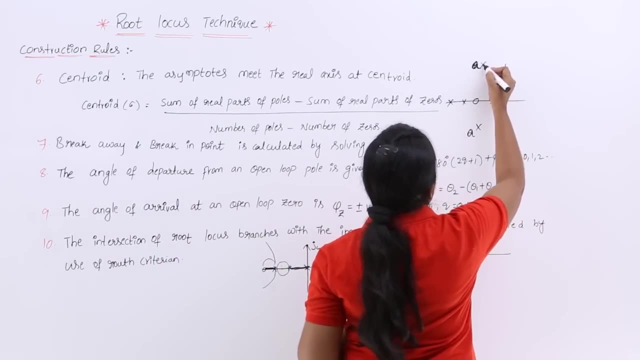 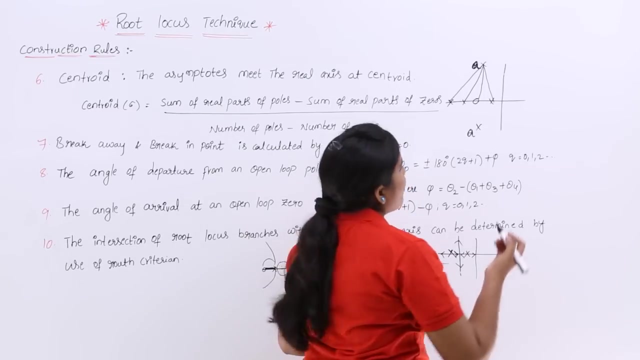 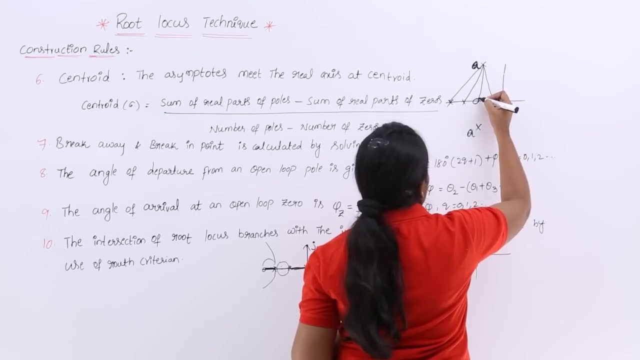 if you are having any pole like this and like this and another pole like this. So how you will calculate means So you will take lines like this, and now here this can be calculated like this: So this is theta 2, this is theta 3, theta 4 and this is theta 2 and this is. 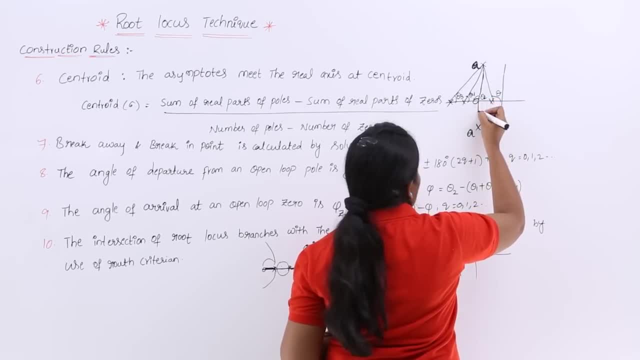 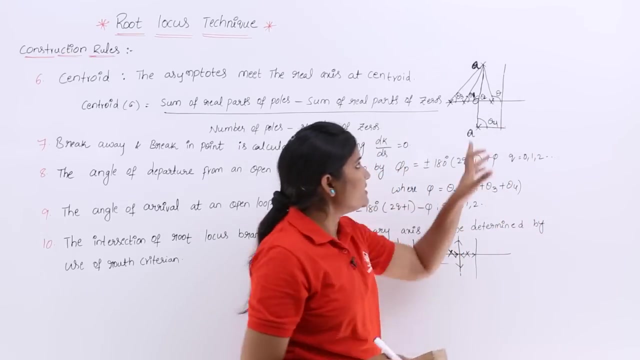 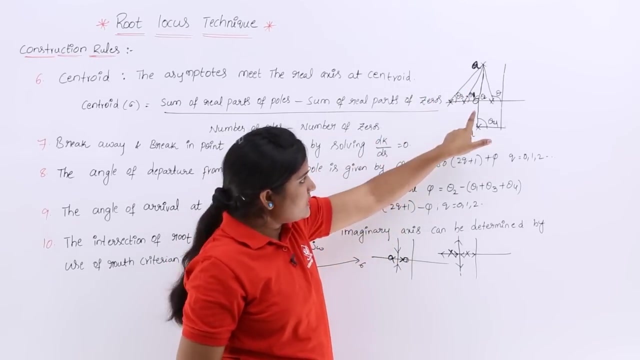 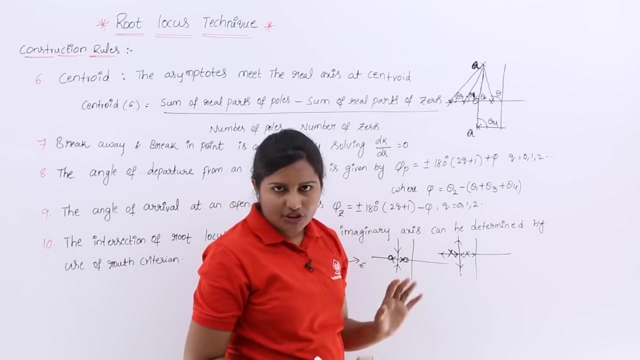 theta 2.. Theta 1: you just consider like any angle. Theta 4: you just consider like this: you can see Now how you will calculate this one Means. So if you want to calculate angle of departure at A, you need to consider this equation In general. we are going to calculate. 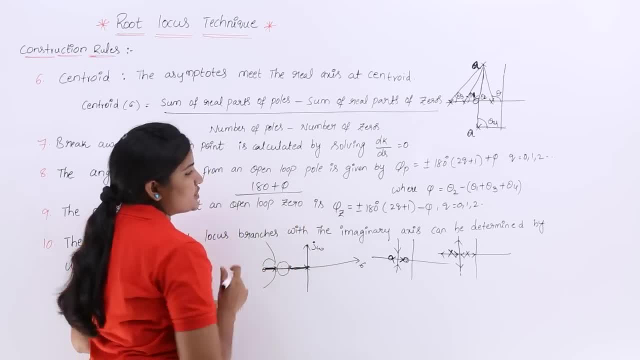 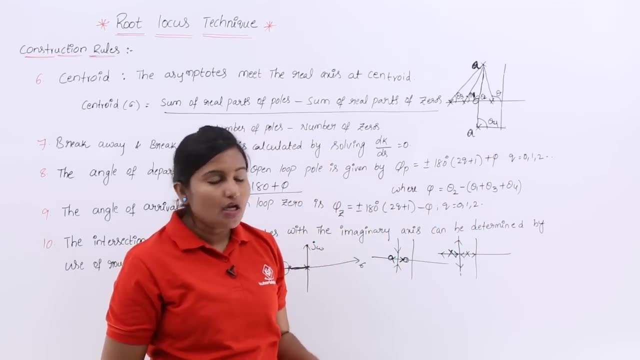 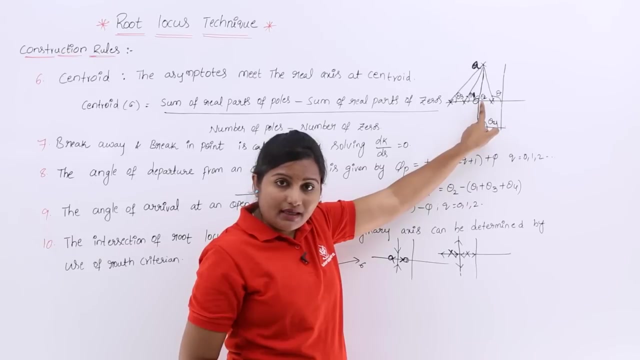 this one, you are going to consider 180 plus phi as the angle of departure. you are going to consider q as 0 and 180 plus phi you are going to consider as the angle of the departure To calculate this phi value. so here, whatever the angle, making by this 0, with this A, that 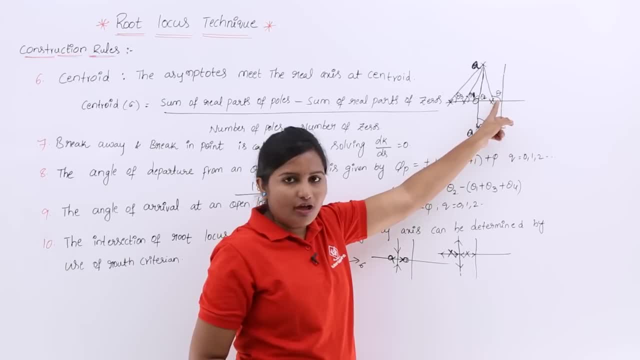 you just consider here, For example, if you are having two zeros, if you are having two 0s, how much angle are you going to calculate everything? Because that comes to be 0, square distance is 0.. Integrity core, so sorry. and then your constant. 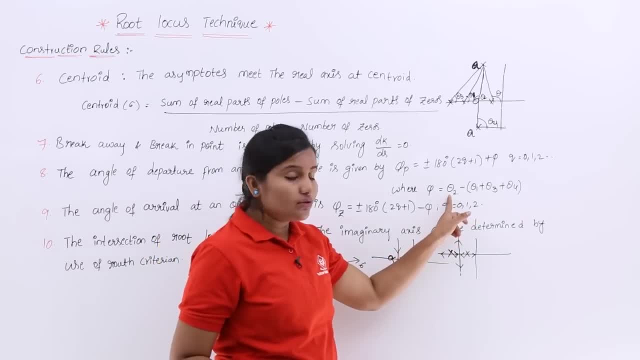 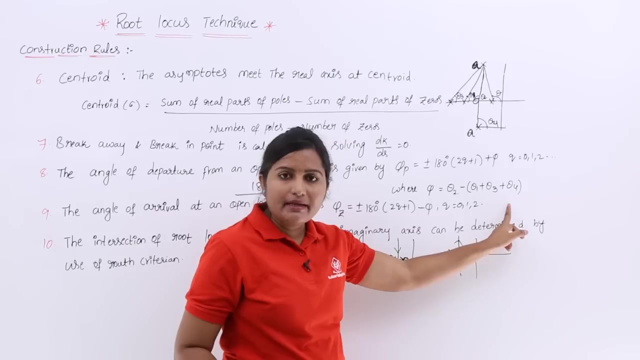 Guesser equation: how much is the along angle of the llevaither концеc of theta To know preço Bolsonaro, How many angles created by that zeros That you will consider here, minus angles created by poles on the real axis. So here phi is equivalent to angle created by zeros minus angles created by. 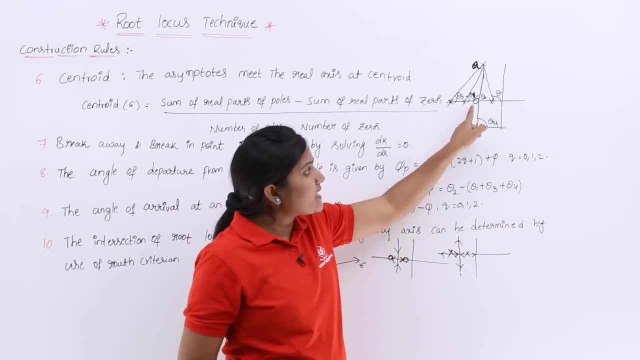 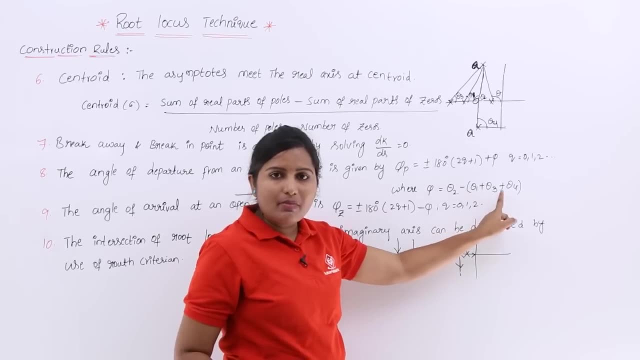 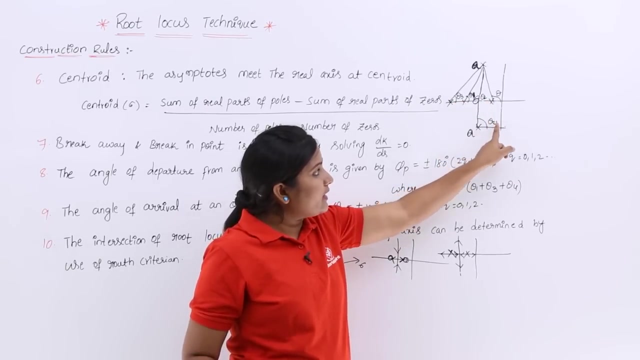 poles, sum of angles created by poles. Here, as I am having only one zero here, the angle created with zero is theta 2 minus the sum of angles created with remaining poles is equal into theta 3 sum theta 1 and here theta 4. I am going to consider like this, For example, if you are: 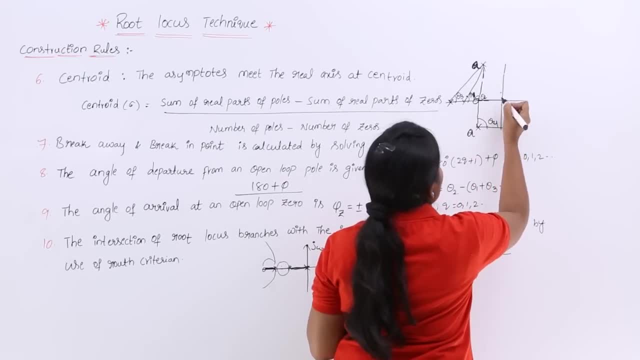 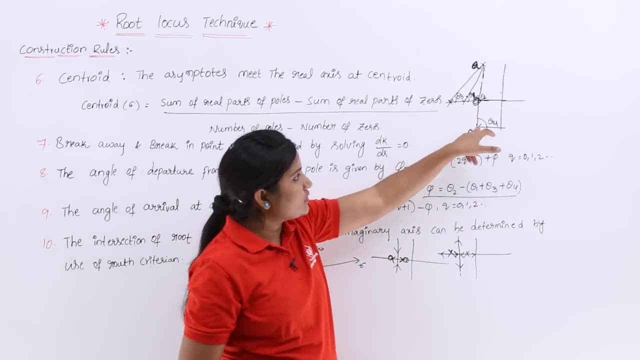 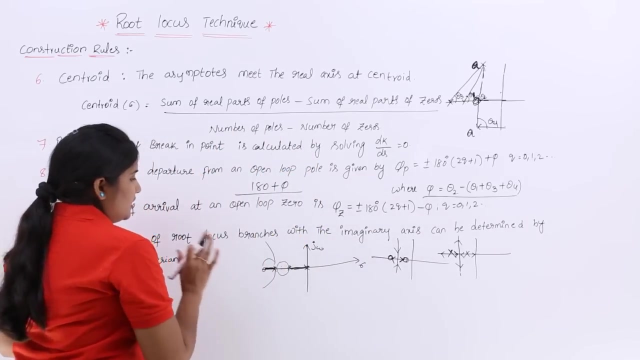 having like this. So here you are, having only two poles and one zero. So this is the equation for the three poles, and so this is imaginary pole Remaining two poles are equal to theta 2, and the remaining two poles is here. So now, here for example, if you want to calculate: 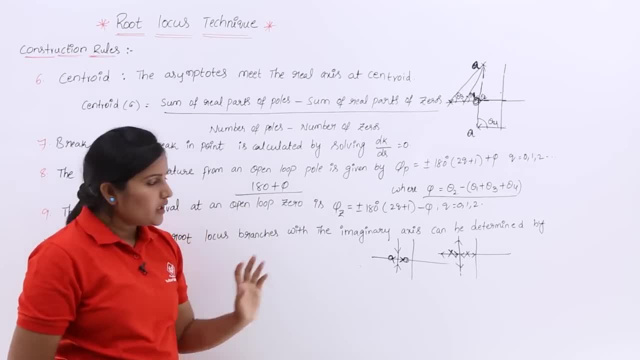 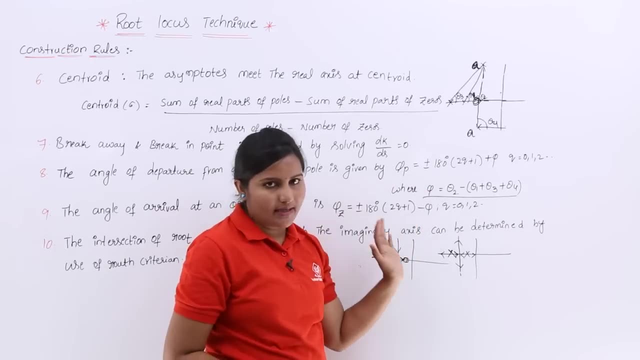 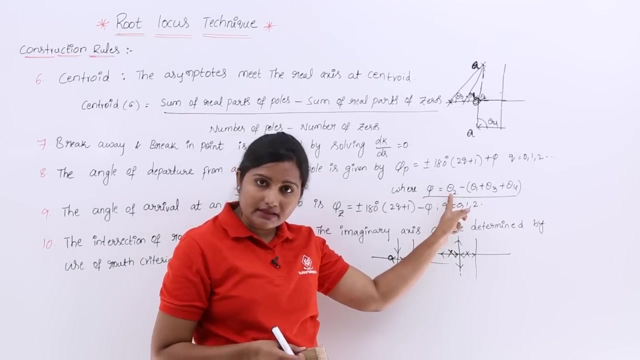 the angle of arrival at open loop 0, then the same equation we are going to use, but minus phi. we are going to use the equation phi will be same. For example, if you are having more number of zeros here, we are going to add that angles made by that more number of zeros 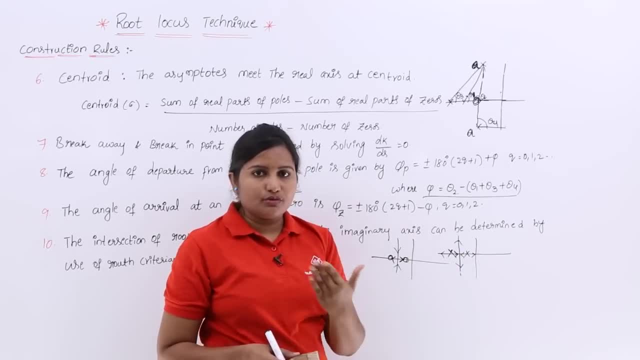 That means, for example, theta 1, theta 2, theta 3, theta 4, theta 5, theta 6, theta 7, theta 8, theta 2, theta 3 are the angles made by number of zeros, and theta 5,, theta 6,, theta 7 or the. 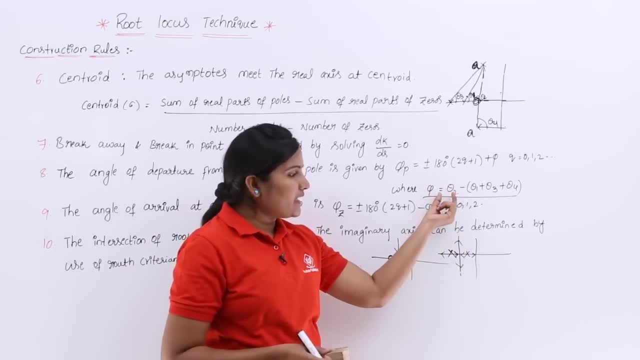 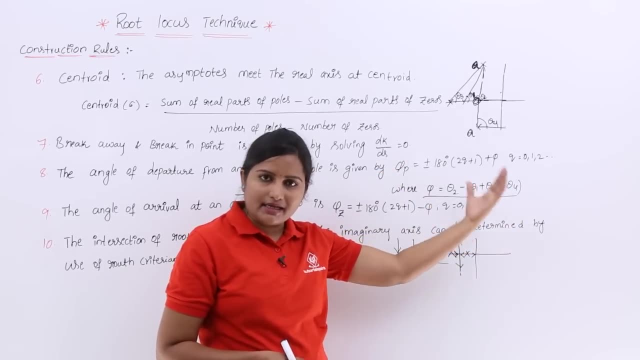 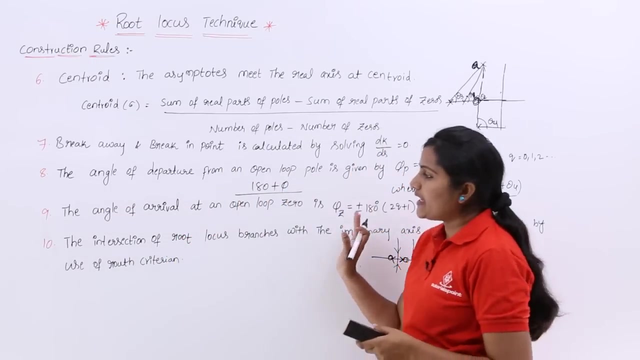 angles made by number of poles. So we are adding that angles made by number of zeros and subtracting the number of poles. that means the angles made by number of poles we are adding and subtracting from this one. So like this, we are going to calculate the 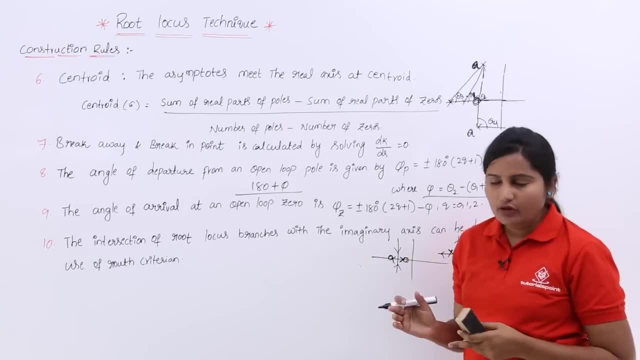 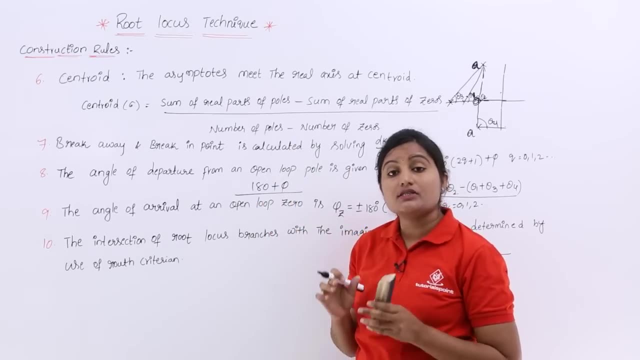 angle of arrival at a point, open loop pole and open loop base, The jednak angle of now let us take, estimated as t, with t theta over t theta 0 at one second Where t legs to the 0. and here the intersection of root locus on the imaginary axis is also very important point. 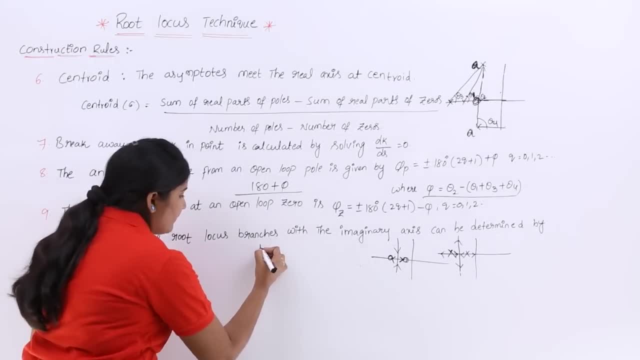 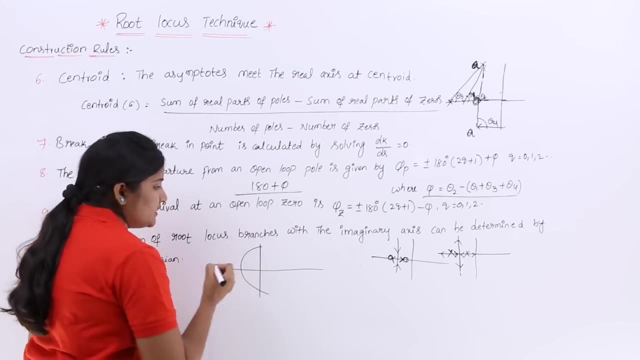 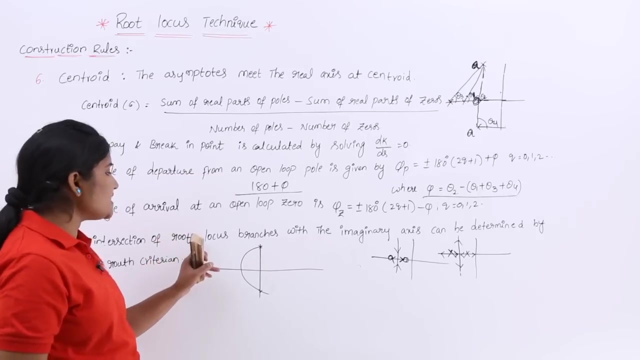 that means here, for example, if you are drawing any root locus, then, for example, if your root locus is like this, then at which point you need to intersect this imaginary axis? that can be decided by the intersection of root locus branches with the imaginary axis. this can be: 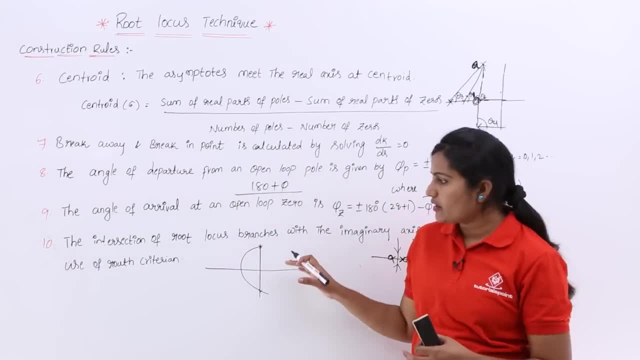 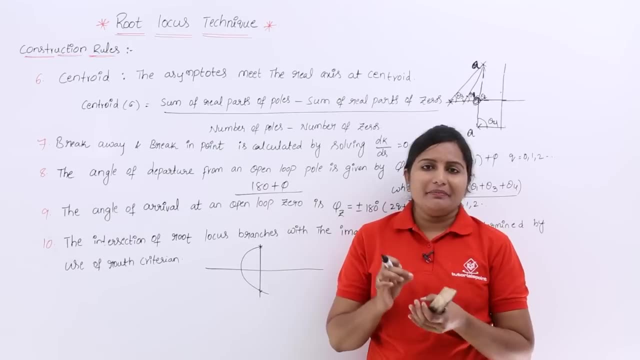 decided by the Routh array. again, we are going to use Routh criterion. So all these 10 points are very important. So what you need to keep in mind when you are drawing your root locus diagram is: so: root locus is always symmetrical about real axis. 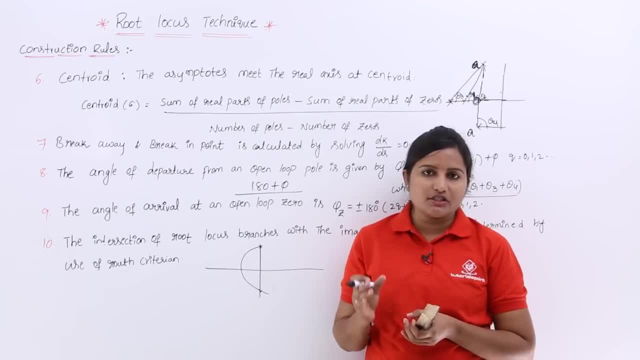 and you need to find out the number of poles and zeros. according to the number of poles and zeros, by taking p minus z or z minus p, you are going to get the number of branches or the number of poles and zeros. So you need to keep in mind that when you are drawing your root locus, 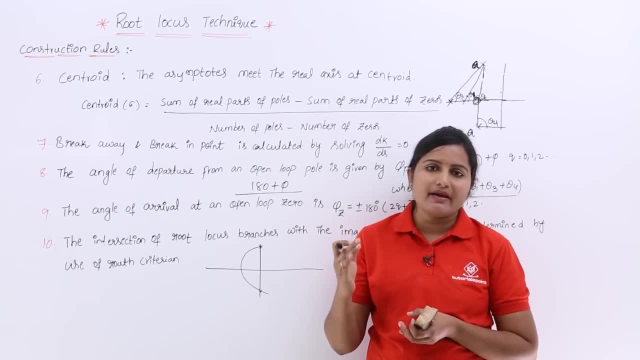 after getting number of branches you need to find out the angles made by that branches or asymptotes. So by using asymptote angle equation. after that you need to find out the centroid- that means meeting point- of that asymptotes on the real axis is nothing but centroid. after that, 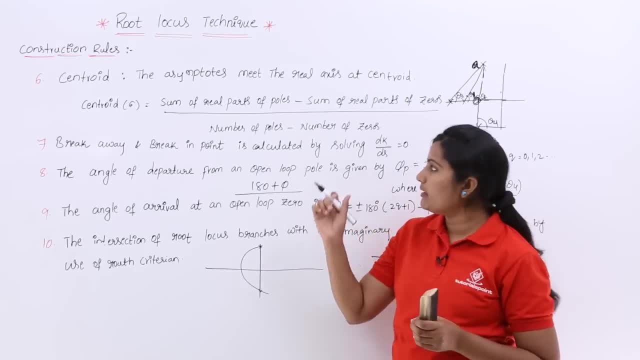 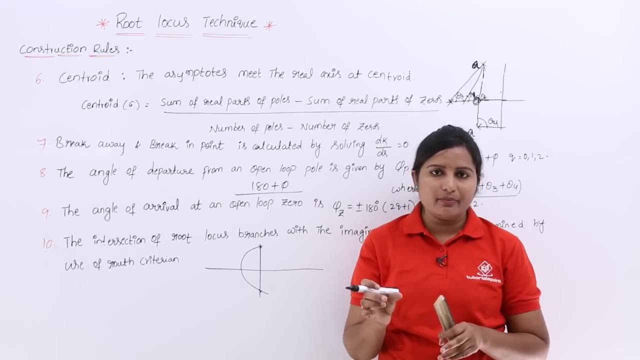 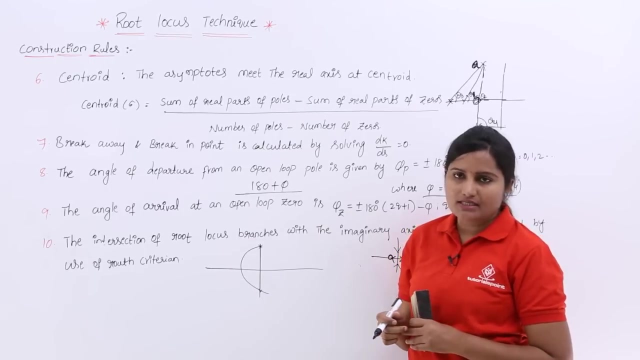 you need to find out breakaway or break in point. by using dk by ds is equivalent to 0. So always in between two poles you may have breakaway point. in between two zeros you may have break in point. So that can be calculated by using dk by ds is. 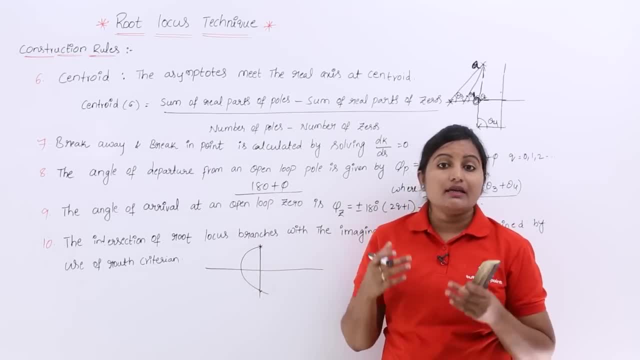 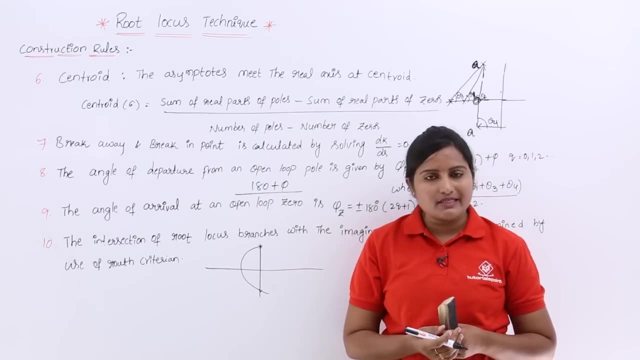 equivalent to 0 the angle of departure. when imaginary pole is there, we will get angle of departure. the equation for angle of departure is equivalent to 180 plus phi, where phi is equivalent to angle made by that imaginary pole, with the zeros on the real axis, minus angle made by that. 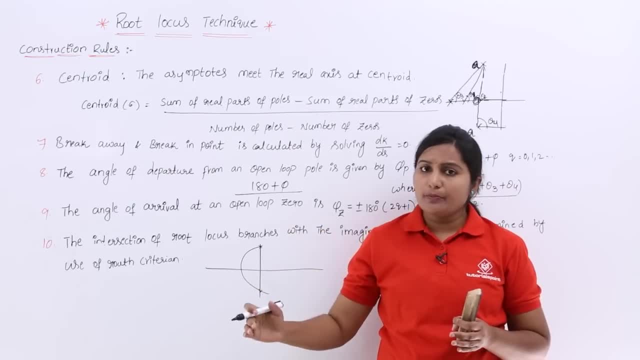 imaginary pole on the real axis. So this is the angle of departure. So this is the angle of departure. So pistol didnot need any animation, may have Ages. how muchigh is it actually similar to 1 by arithmetic Poles of pointae, alpha and niew圧 times, single Lenovo. 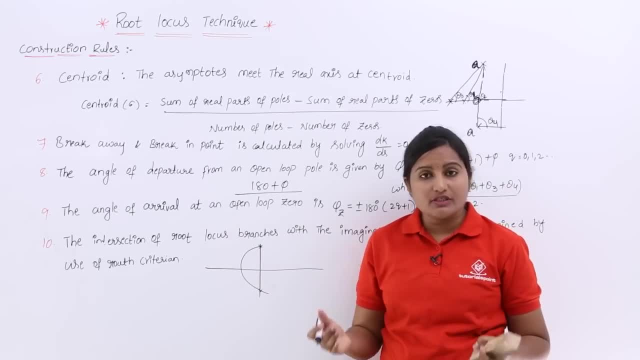 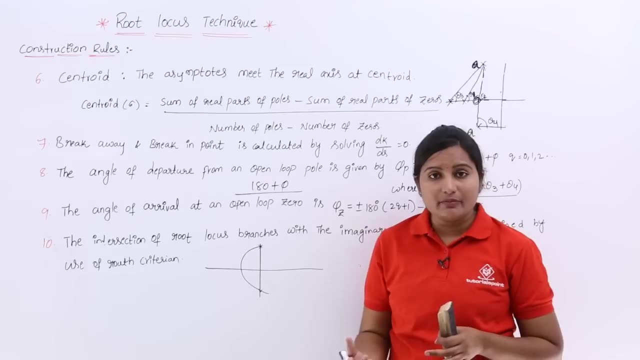 multiplicity to the poles on the real axis. So now, similar to that, the angle of arrival at an, the open loop 0, if you are having any imaginary open loop 0. So here the angle of arrival will be there. the angle of arrival is equivalent to 180 minus phi. again phi is equivalent to: 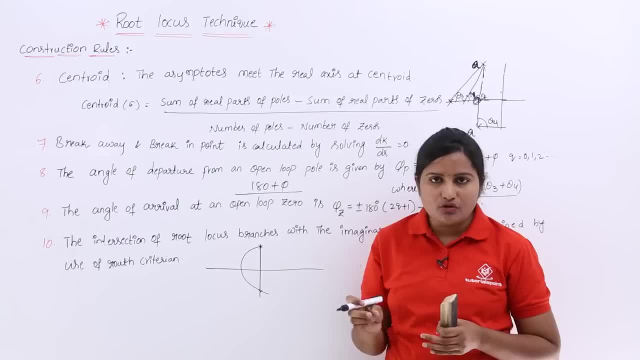 the angle made by that open loop 0 with the zeros on the real axis, minus angle made by that open loop 0 to the poles on the real axis. So finally, we are having intersection point of the root locus on imaginary axis, Intersection point of root locus on. 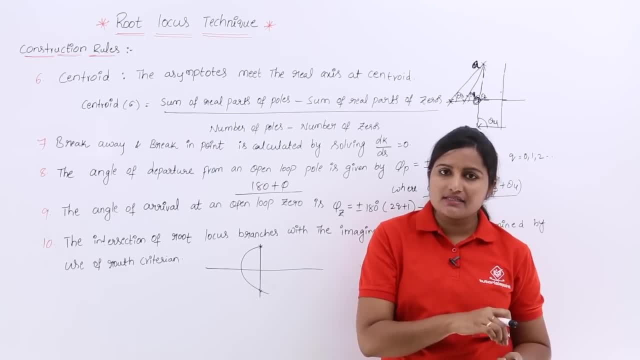 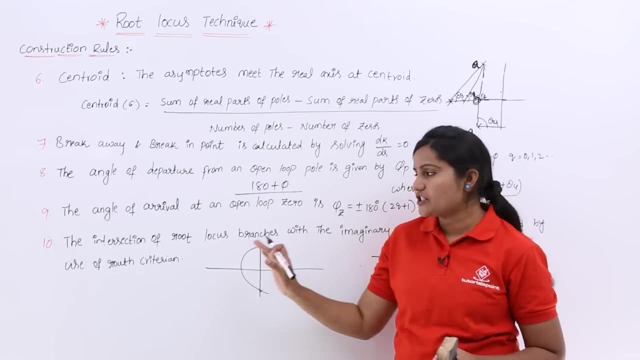 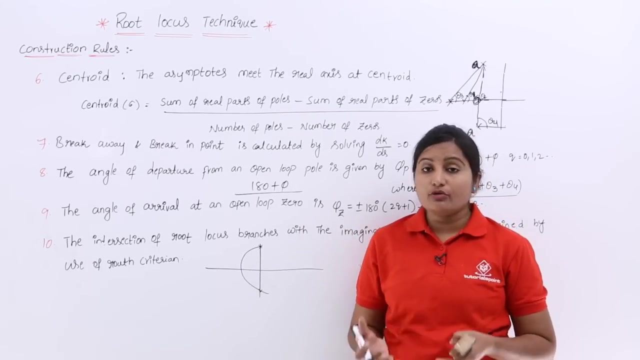 root locus or asymptotes on the real axis is nothing but centroid Intersection point of the root locus on the imaginary axis is nothing but intersection point. This can be determined by the Routh Hedge criterion again. So by solving one problem you are going to clear so many problems. 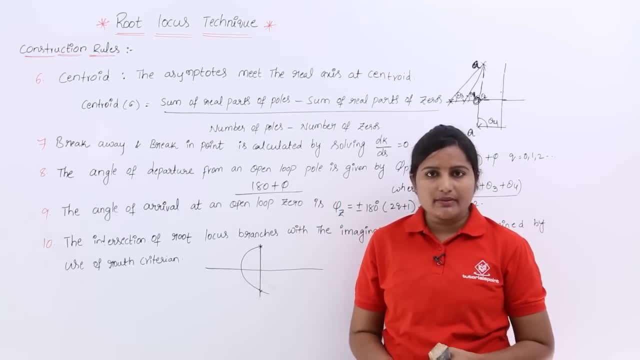 related to this constructions rule. So in next step we will see the problem related to root locus technique.